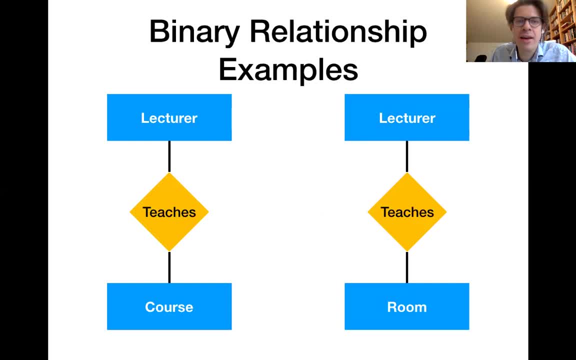 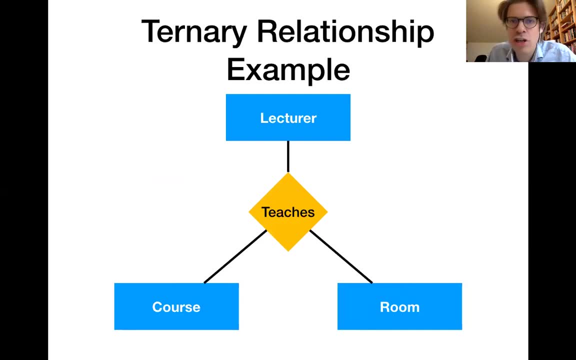 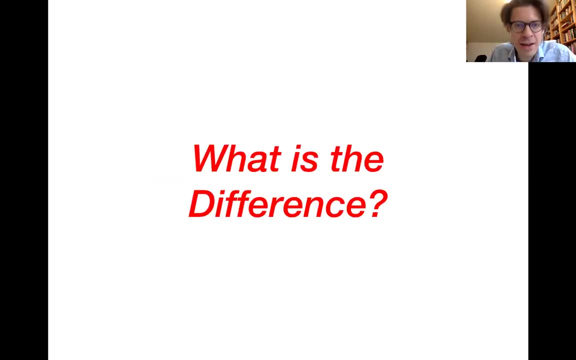 those are binary relationships because they connect two entities. All right, we can also have ternary relationships connecting three entities, or even relationships that connect more than three entities. There is some differences in terms of the semantics, in terms of what you can model. 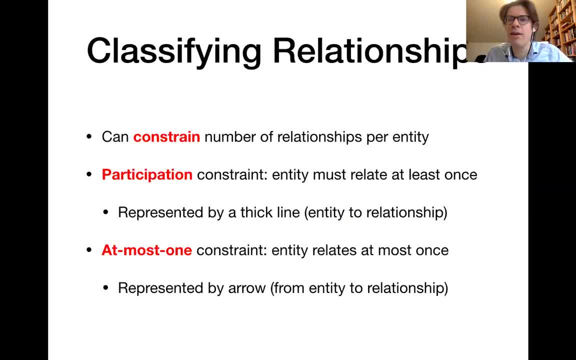 with them and we have quickly discussed about that last time. We have also seen that the data set we've used in the universe can be more or less consistent with those that we've also considered. This is a well-studied example, So, like I said earlier, we can classify those. 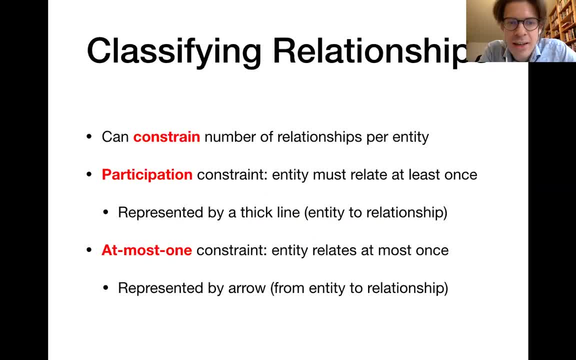 relationships further by introducing a constraint. In particular, we have seen the participation constraint, which essentially means that an entity needs to be related according to a specific relationship with at least one other entity, and the at most one constraint essentially means that in a binary relationship or, for instance, in a ternary relationship, it can be related to at. 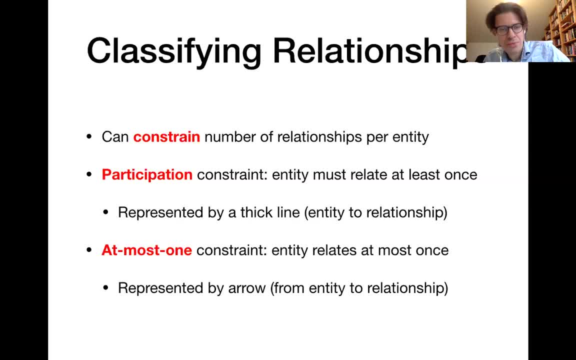 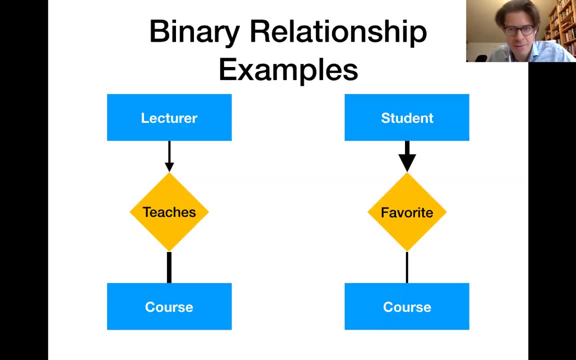 most one combination of entities. So we represent participation constraints by very thick lines in the diagram and at most one constraints are represented as arrows in the diagram. So this is an example here. For instance, on the right-hand side of the slide we have the example that, as 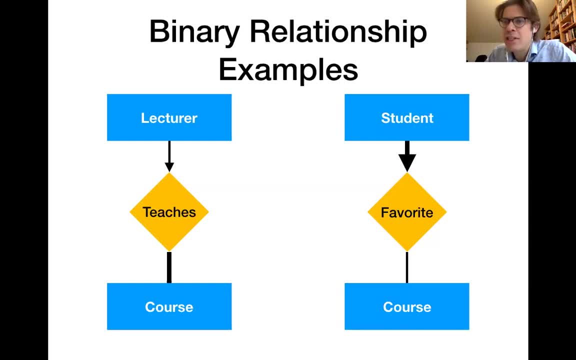 students. they have one favorite course, and here you see the combination of a participation constraint and an at most one constraint, because here we have a thick line and an arrow, meaning that each student is linked to exactly one course that is the favorite of the student. 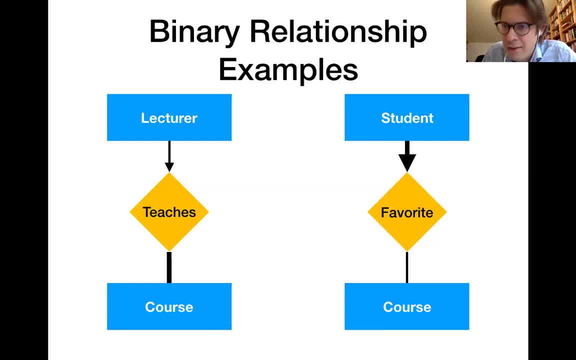 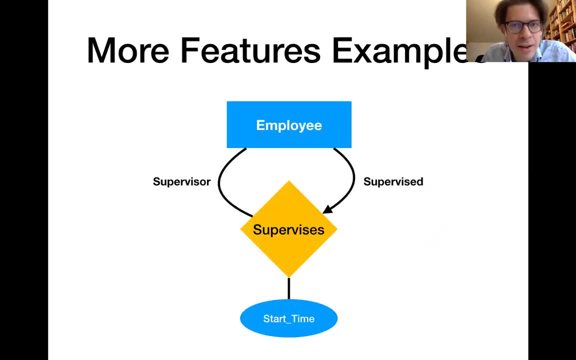 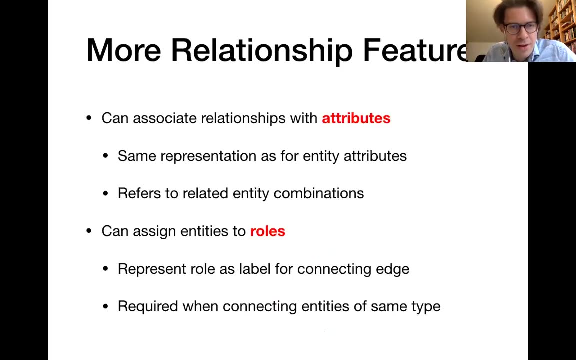 So this is how far we got the last time, and then we have started discussing about the classes, Then we have started discussing about subclasses. So maybe I should also very quickly remind those two features. So here we have also quickly discussed about the fact that we can 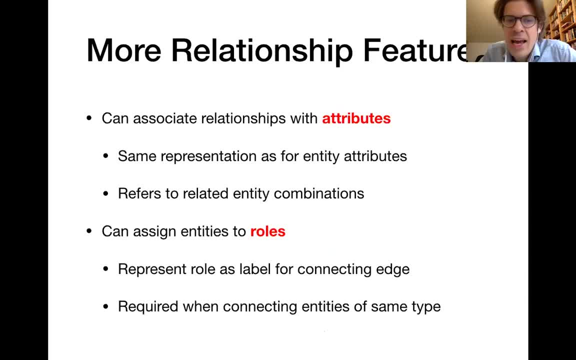 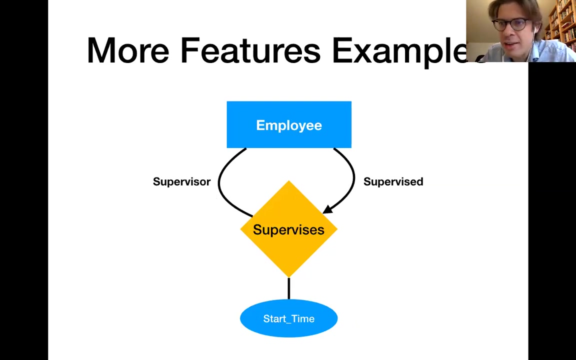 associate relationships with attributes, and also we can associate relationships with roles that we assign to the different entities that appear within a relationship, which is very important. So are required in cases where a relationship connects entities of the same type. Perhaps here let's have a quick look at this example again. So here, 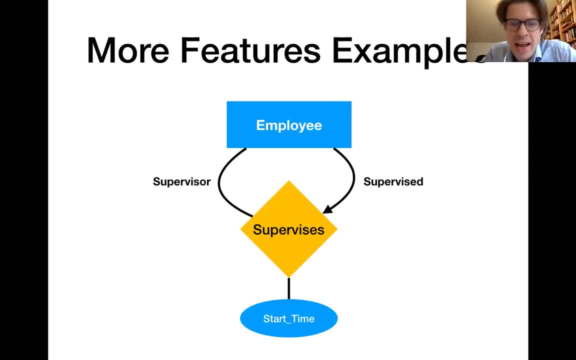 we have the entity of type employee and there is a supervisor's relationships between different employees, which is associated with an attribute. that's the start time of the supervisor's relationship. So, starting from when was this employee managed by this other employee? And here we have a relationship. 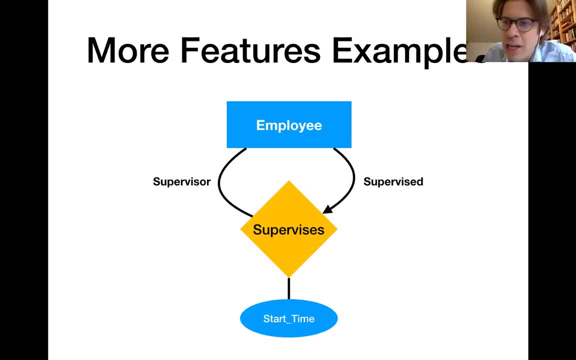 that connects employees together. so we are connecting entities of the same type. and then becomes important to assign those entities to roles. and here you see, those roles are modeled as labels on the lines connecting the relationship to the entity type. You have the supervisor role and we have 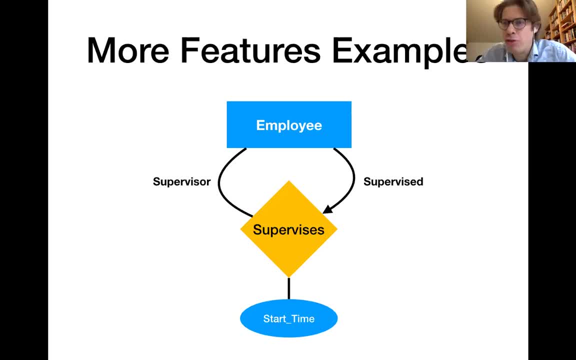 the supervisor role and the supervisor role Ao. you see some of these roles being role. There's also constraint in here, as you see, based on the arrow. So for the supervised employee we can have at most one such relationship, So each employee can be supervised by at most one supervisor. So that is a little reminder. 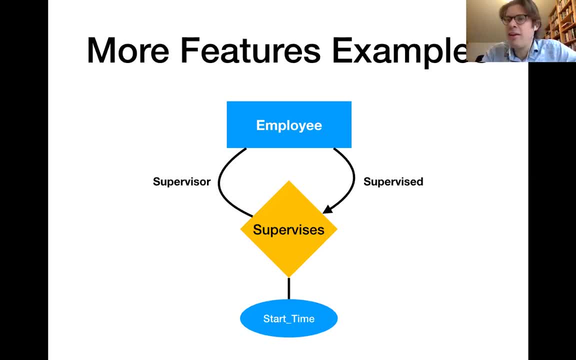 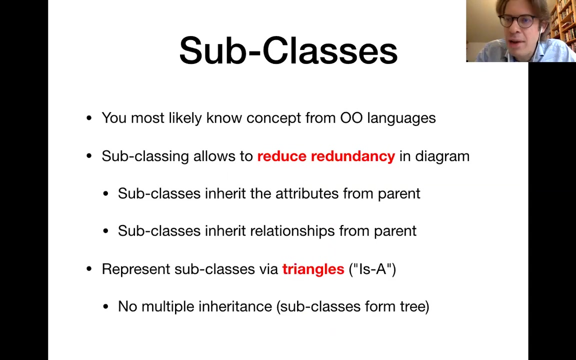 of the things that we have seen and on the following we're going to see more features of entity relationship diagrams and later we will see how we can translate those entity relationship diagrams into actual SQL commands or into relation schemata. So one feature that entity relationship diagrams allow. 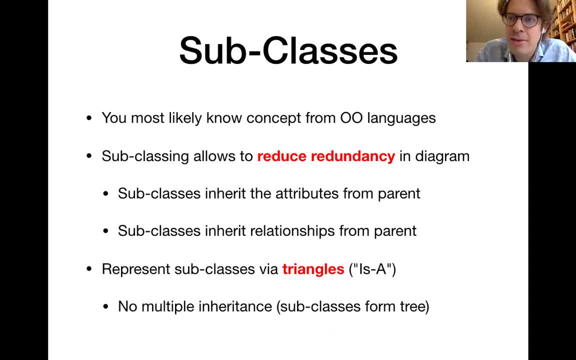 to model is subclasses, which is something that most of you might already be familiar with from object oriented languages, and, And if you introduce subclasses in your diagram, you essentially reduce the amount of drawing that you need to do, because the subclasses automatically inherit certain things from the parent class, such as the attributes and also the relationships. 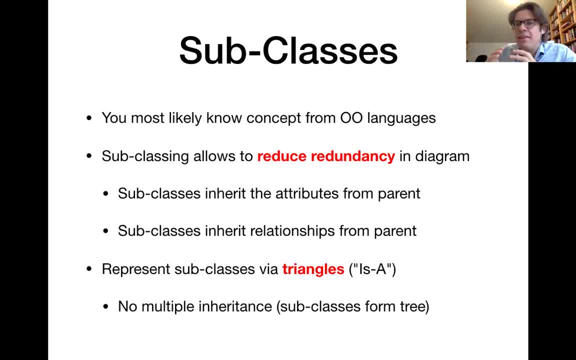 So if you say that one entity type is a subclass of another entity type, then you save yourself the work of having to redraw all the attributes that are in common between a subclass and a superclass. We represent those subclasses as triangles, Those triangles, they're connected to the superclass and to the subclass. 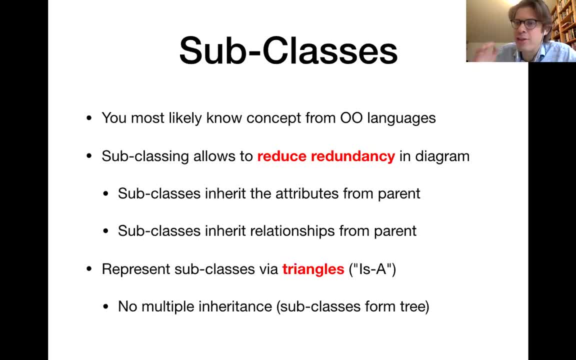 And typically still have some label. So inside of them, for instance, there is a label: We only support, we don't support multiple inheritance. So if you only consider those subclassing relationships between entity types, then that will form a tree. 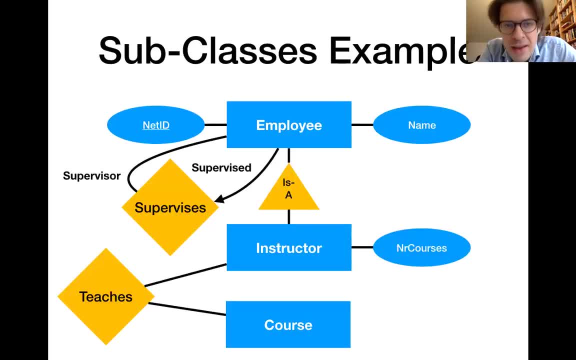 To make things more concrete, here is an example. And let's, for instance, assume that we have a university database, So we have employees, And then perhaps there's different classes, So we have the classes of employees, such as the instructors, and to hear the employee already has a couple of attributes. 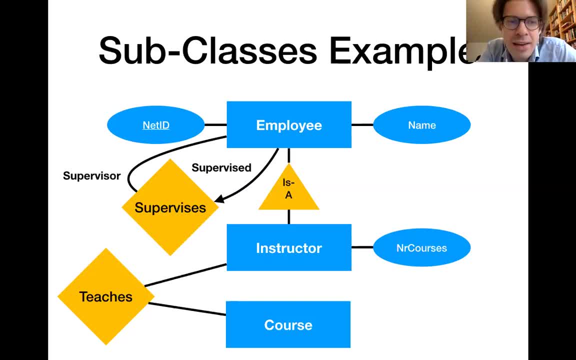 So, first of all, we have the net idea, and the net idea is a key at which you recognize because it is underlined. We also have the name attribute, and those employees are also in a supervisor's relationship with each other, which we have seen in the previous example. 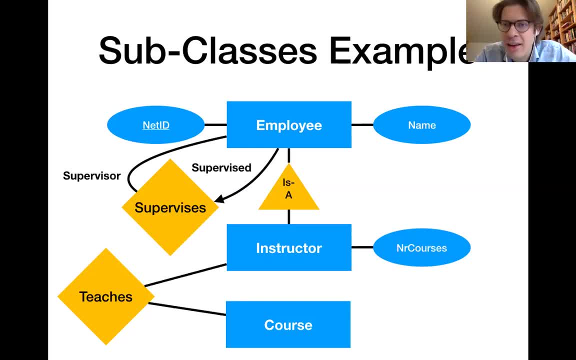 And now we essentially introduce A specific class of employees, which is the instructors, and we can represent that using the subclassing relationship. So you have to is a relationship and it connects the employee to the instructor and the instructor is thereby classified also as an employee. 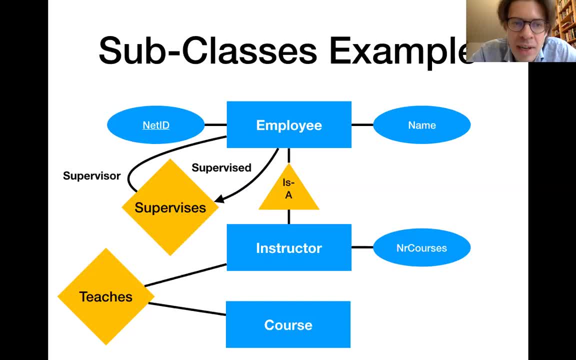 So it will automatically inherit the attributes net ID and name, even though you don't see them here Explicitly in the diagram. it also adds a new attribute, which is the number of courses, which only makes sense for instructors but not for other employees. 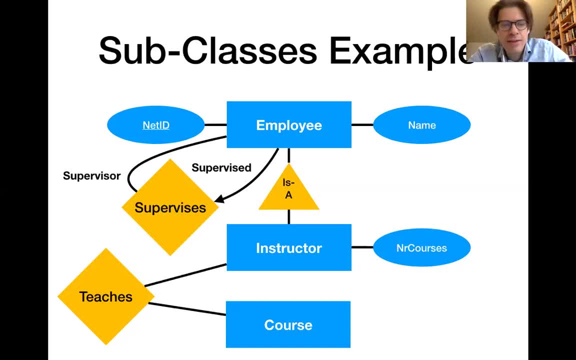 And it also adds a new relationship, which is the teacher's relationship, which connects an instructor to the courses that are taught by this person. So here we have added a relationship and a new attribute that only makes sense for this specific subclass of entities. 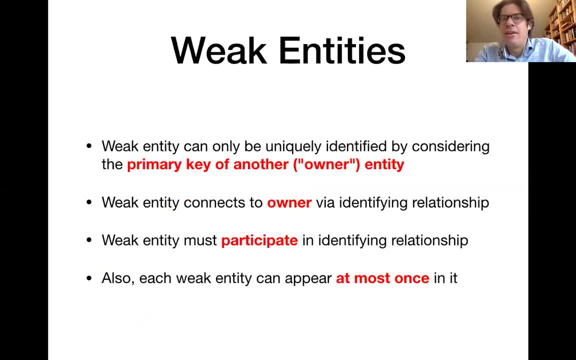 Now another commonly used a feature in the context of entity relationship diagrams. this is a weak entities, And a weak entity is generally an entity that cannot really stand all by itself. It's always dependent on another entity and we call that other entity the owner entity. 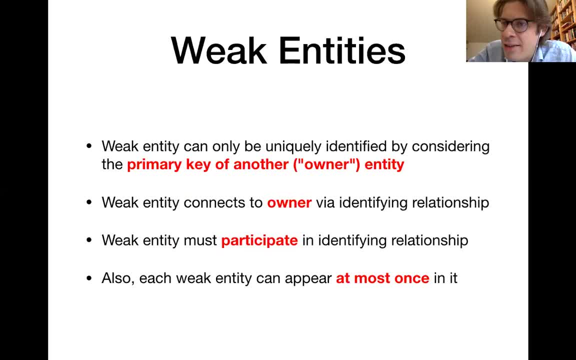 So, more precisely, the weak entity, We'll have some primary key which essentially only becomes unique if you combine it with the primary key of the owning entity in order to indicate which is the only entity. we have to connect the weak entity with a relationship to the owner entity and it has to be a specific type of relationship. 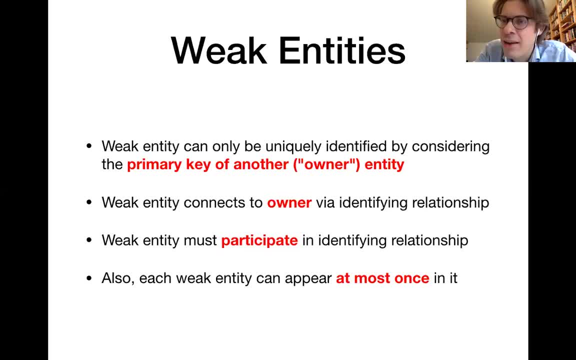 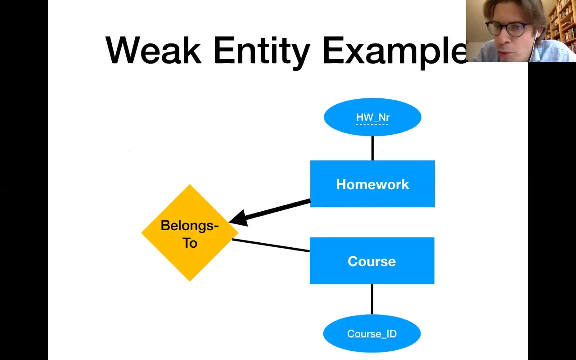 The weak entity Needs to be connected by an exactly one relationship to the owning entity. And to make things more concrete, Let's just look at an example. So here, for instance, assume that we have an entity type homework, which stores an attribute, that is the homework number. 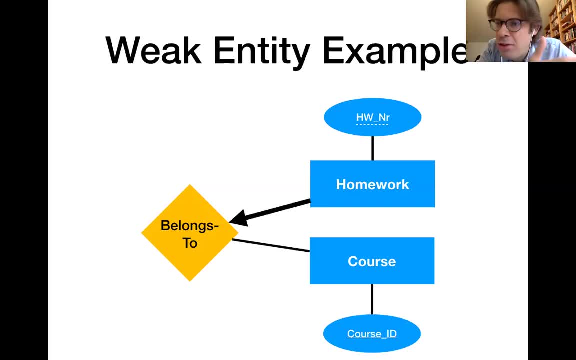 And the homework number all taken by itself is not necessarily unique, because a homework could belong to different courses, So there will be a homework one from multiple lectures. So as long as you only store the homework number, it doesn't uniquely identify the entity And this is indicated by underlining the homework number here by this dashed line. 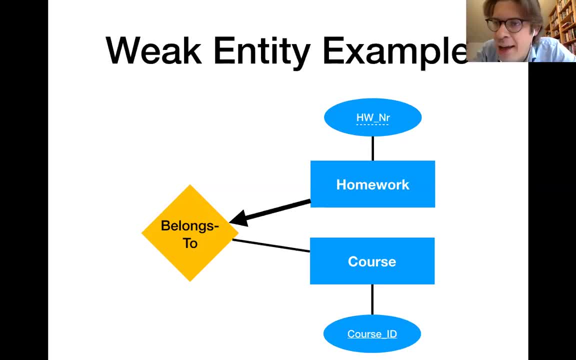 So this is different from the non-dashed line that we use for primary keys. So here the homework with the partial keys, The key homework number, is connected via the belongs to relationship to the courses table, which has the course ID primary key. And now if you take both of them together, if you take the homework number and the course ID together, then you get a unique identifier for one specific homework. So that is the semantics of the weak entities. 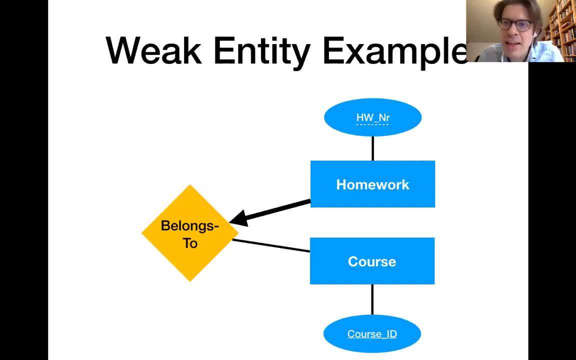 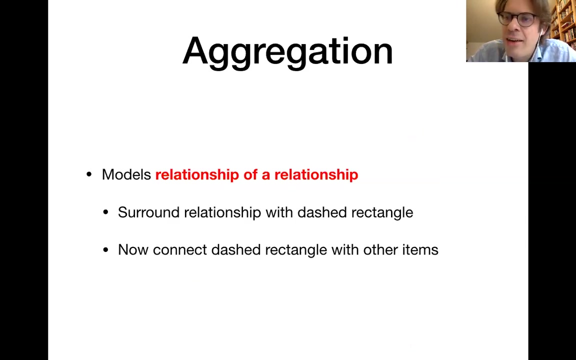 They don't have a really unique key, but if you combine their key With the key of the owning entity, then you get a unique key, And here, in this example, the weak entity is the homework. Another important concept in the context of entity relationship diagrams is aggregation, And that essentially models a relationship of a relationship. So if a relationship between entities exists, 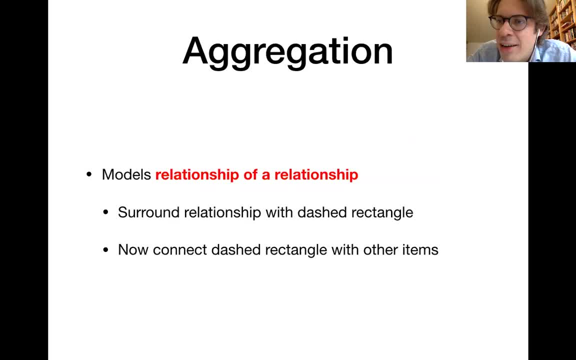 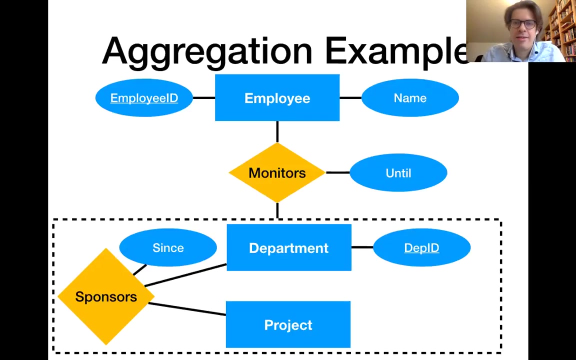 then you get a unique key. We can add some additional information about that. We represent this by putting the first relationship into a dashed rectangle which contains the relationship and the associated entities, And then you connect this dashed rectangle with other items. This is how it looks like. So here, for instance, we could have a situation in which we have: 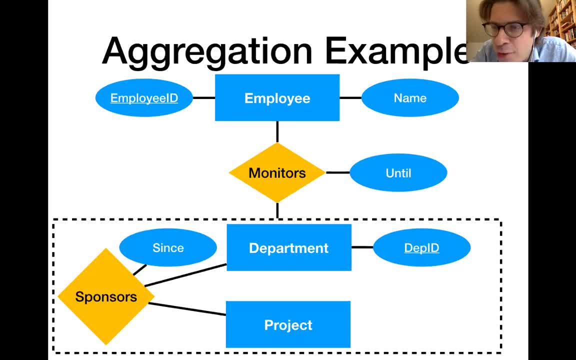 departments associated with a department ID which is a sponsor project, And this sponsoring relationship is associated with a since attribute, meaning this is the point in time at which the sponsoring started. And then we have employees that monitor this sponsoring relationship, making sure that everything is accounted properly. for instance, 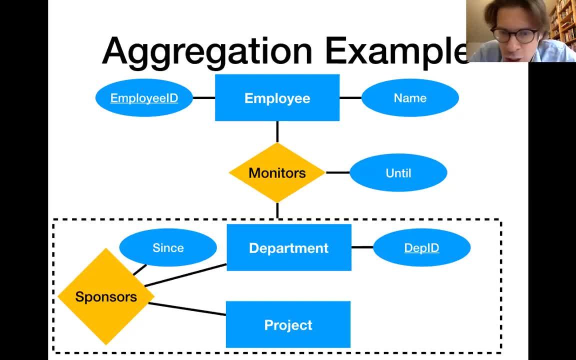 So this is why we have two departments, aggregation relationship. So we have put the first relationship, the sponsoring relationship, into a dashed rectangle and now we connect that relationship with corresponding employees that monitor the sponsoring relationship. So here we have the monitors relationship, which is relationship. 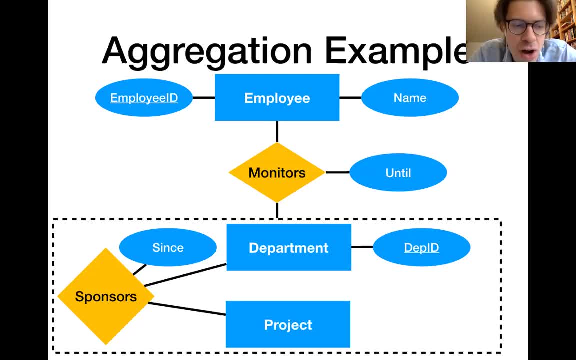 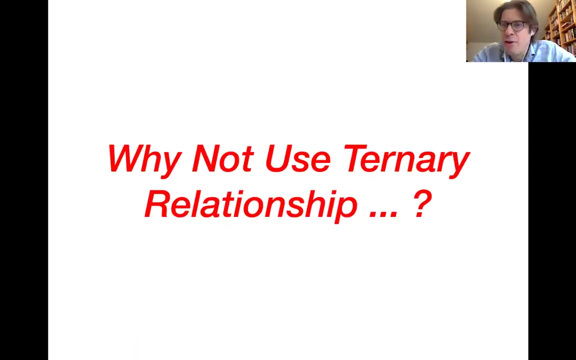 connecting employee entities to sponsoring relationships. So that is aggregation. And perhaps to clarify things, I mean in this situation, you could also imagine that we are connecting perhaps three entities: the employees, the departments and the project. Does anyone have a suggestion about reasons why we would prefer the? 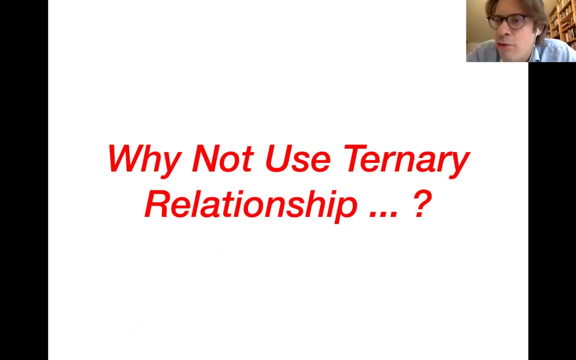 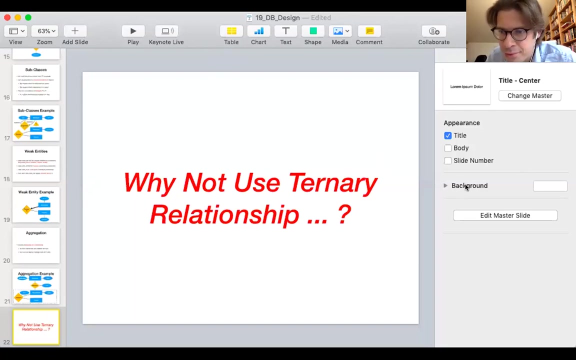 aggregation relationship. So here we have the organization in some cases over those ternary relationships, And here you see the Liverpool, see the List of Non-L не results for each of the positions, So it's very OK. So there is the proposition that the department might be monitoring mache zur. 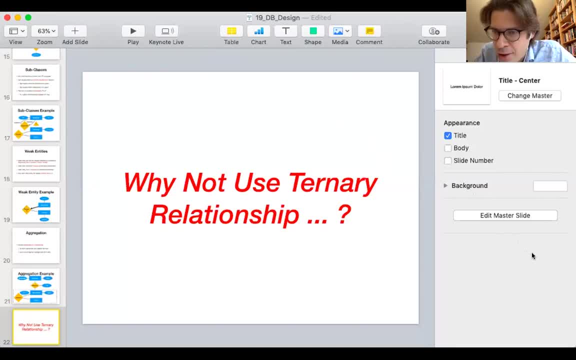 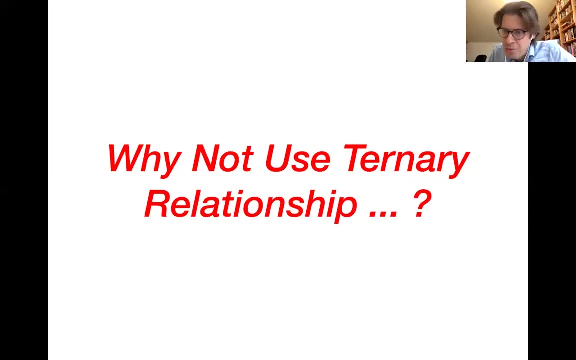 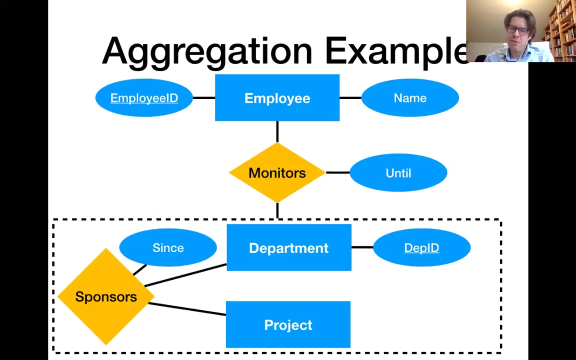 multiple projects and we don't want to repeat employee every time when we are drawing. so you have multiple propositions coming in. so here the money to us. relationship connects one specific employee with one specific combination, essentially between department and project. mm-hmm. you, if you think, for instance, about the constraints that I could add here. 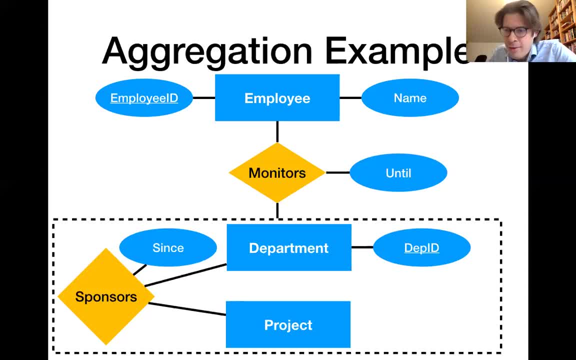 so this all goes into the right direction already. I mean, there's many reasons or ideas, multiple correct replies and specifically thinking about a case where I want to introduce constraints on those relationships if you imagine the same thing, if you imagine, instead of this, a tannery relationship. 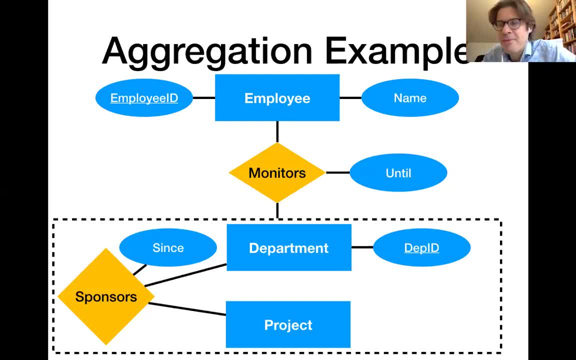 between employees, departments and projects. you now okay, yes, very good. so now, yes. So here the proposition is to look at those constraints on relationships that we have seen Here we have at least one relationship mentioned, and there's also the participation constraint mentioned. So here, for instance, what I could model would be something like making sure that each combination of a department and project. 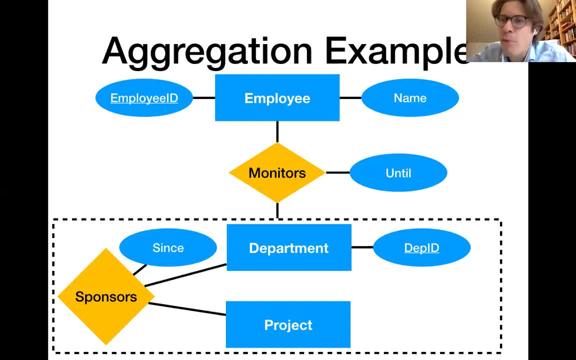 where the department sponsors the project is monitored by someone. So I could express this by a participation constraint that connects the sponsor's relationship to the monitor's relationship. Now, on the other side, if you have a ternary relationship, you might be able to express that specific departments or specific projects can get monitored. 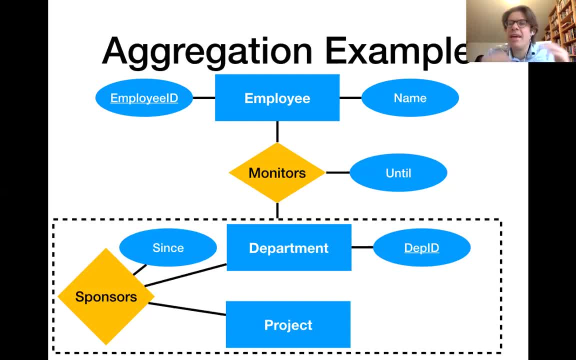 but you cannot really express that. the combination of a department and a project needs to get monitored, And that is only one example. So here we could have multiple constraints that we can model when having two separate relations, but we cannot model them when only having one ternary relationship. 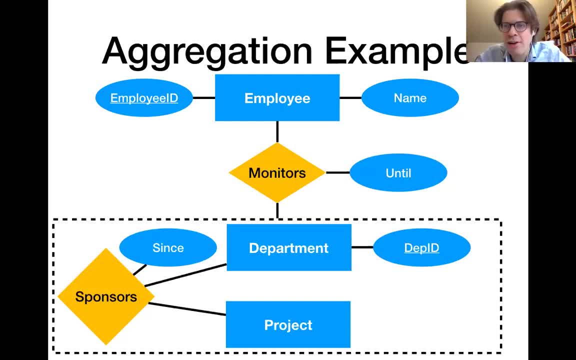 So there's a lot of subtleties about which model, which entity relationship diagram, you choose in order to model a certain situation, And you have to be careful that whatever representation you choose really allows you to model all the constraints that you want to add. 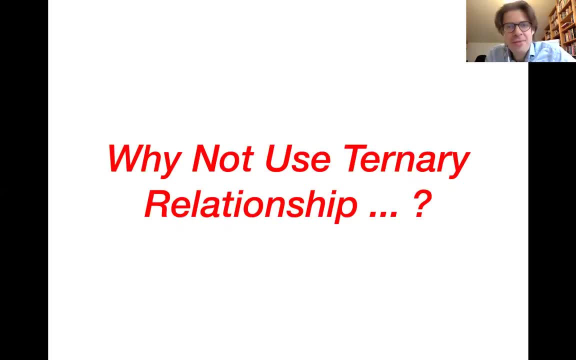 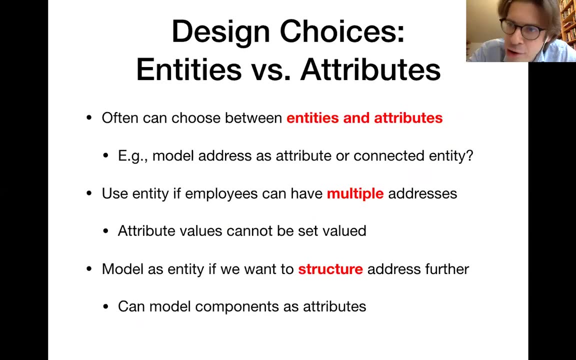 Okay, So very good propositions here, All right. So in general, you have a couple of design choices Now. here we have already discussed aggregation versus ternary relationships, And one thing that you also often can choose is whether you model certain things, either by introducing new entities or by adding attributes to an existing entity. 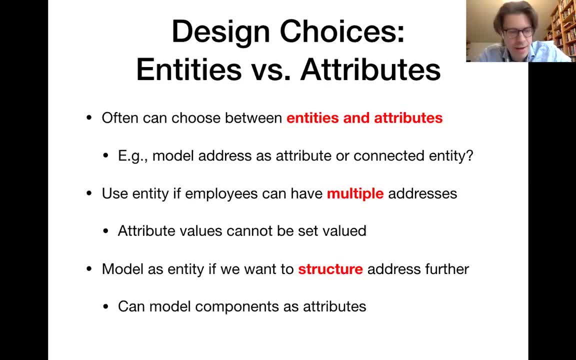 For instance, if you think about something like an address. let me quickly move something here. If you think, for instance, about an address, then you can either consider introducing an address entity or you can consider this rather as an attribute of an existing entity, like of an employee. 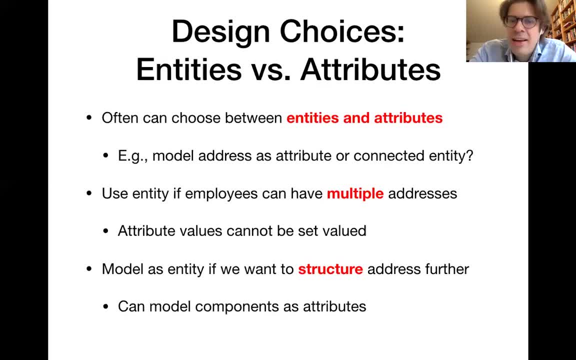 The first thing to consider is whether the entity, for instance the employee, can be associated with multiple addresses, Now attributes in entity relationship diagrams. they must have simple types. They must have, for instance, string or integer types. In each case, they cannot store a set of values. 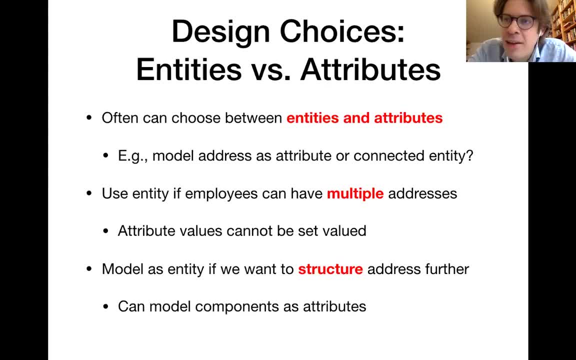 They can only store a single value. So if you want to model something like one employee could have multiple addresses, then you have to model this by an entity as opposed to an attribute, because those attributes they couldn't store a set of addresses. And also if you want to structure the address further, 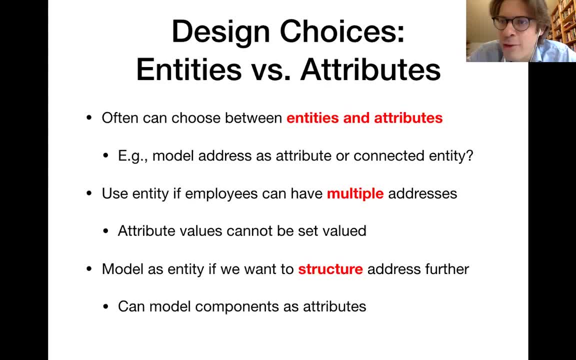 so often like, an address is structured into multiple fields. you might have the street, the street number, the city and so on. If you want to represent that structure, then you also have to model it by introducing a new address entity, Because then you can model those different components. 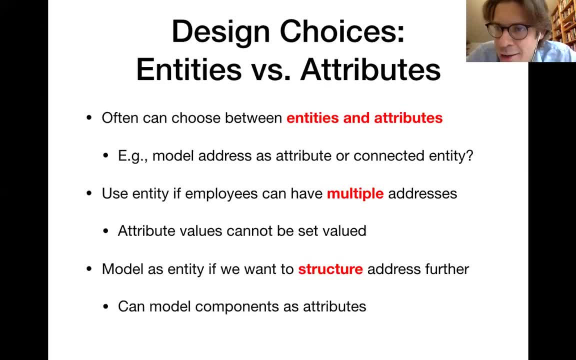 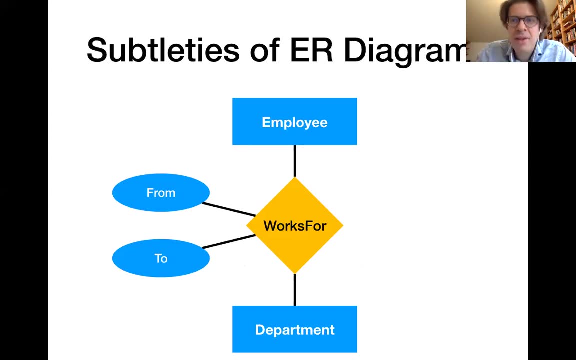 as attributes of the address entity. So those are some of the things to consider when choosing between entities and attributes in your model. Here we have an example. What we are modeling here is the works for relationship between employees and departments, And this works for relationship. 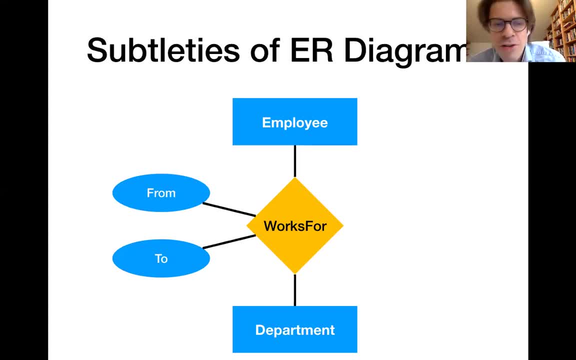 between the two attributes. So the work for relationship between the two attributes is associated with two attributes: the from and the to attribute. Can anyone tell me what might be wrong with this representation? Can you imagine a situation that you would like to model? 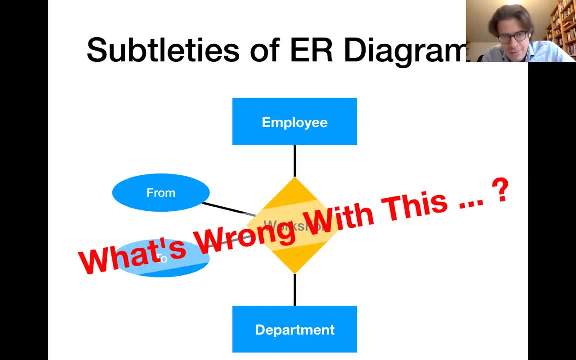 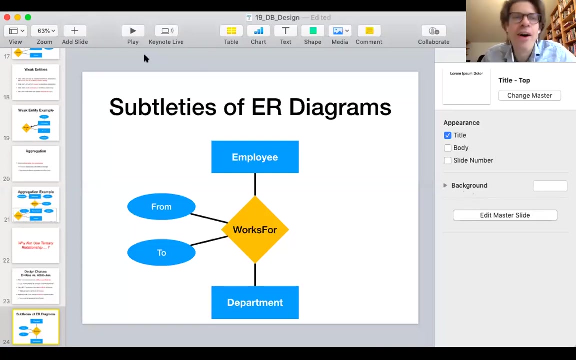 but cannot model with this representation, So I'll remove the questions so you can see the diagram better. And here you can see what might be wrong with this representation. Okay, very good, And here is exactly the point that I was looking for. 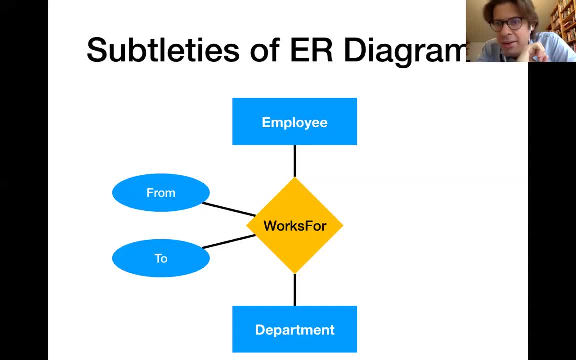 Great. So the thing is this: One employee might work with two other employees, And so, for example, I have a company of two employees And I want to work with them repeatedly for the same department. Maybe that person worked for a different department. 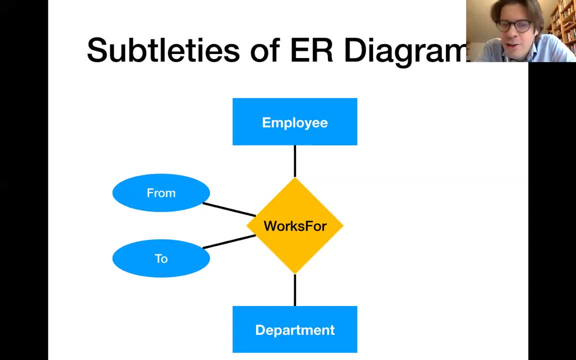 for a while and is coming back to the first department, or even work for a different company for a while and is coming back to the department, And that means that I want to be able to associate one employee with a multiple time periods during which the employee worked. 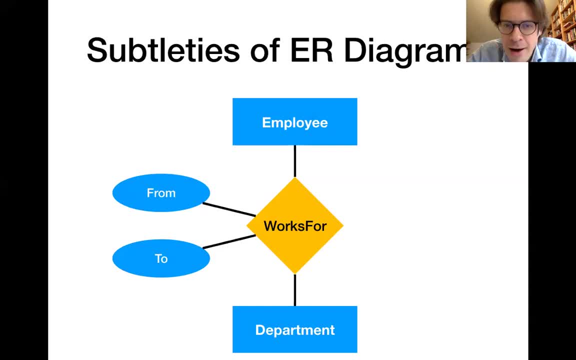 for one specific department. Now, in this representation and the two attributes, they have a one value for each: a combination of an employee and a department, right? so here the works for relationship connects one employee and one department, and here we can associate works for with from and. 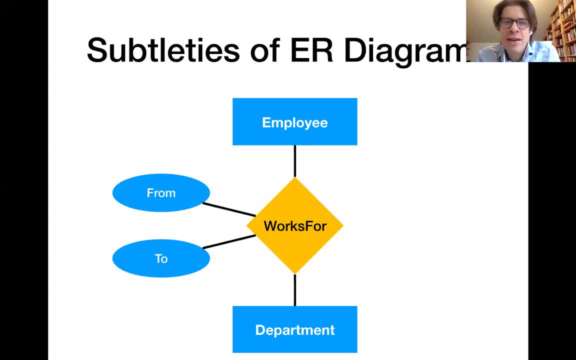 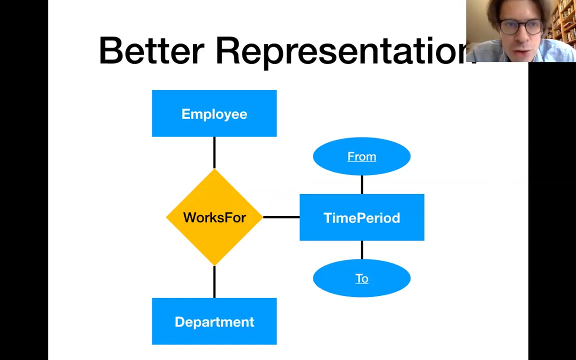 to. but we can only we can only pick one value for from and to for one specific combination of employment and of employee and department. so if you want to resolve that, a better model would be the one that you see here. so here we add a new entity type. 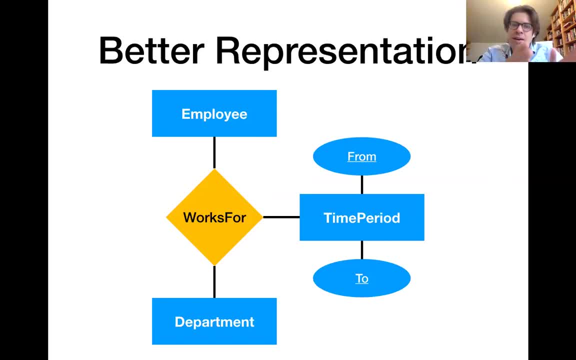 time period of the employment. and then we model the works for relationship as a tannery relationship connecting employees, departments and two time periods. and for the time period- here we can, we can introduce again the from and to attributes. and so here, for the same combination of employee and department, 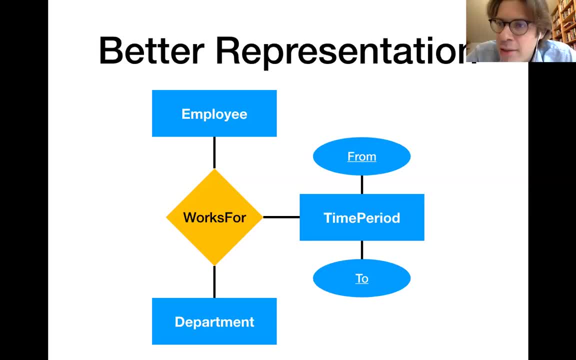 we might actually have multiple time periods during which the employee work for the department, right, so that is somewhat subtle points, but then creating a database, then those points actually matter a lot and you have to be very careful that all the constraints that you want to represent and all the things that you want to be, 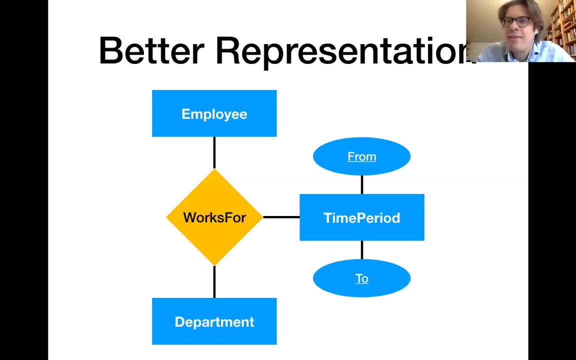 able to express can be expressed using the database model that you are choosing. is there any questions on this? okay, that's an interesting proposition. so we, the proposition is that we might also consider using aggregation here. so we have the employee and the department, that is the works for relationship, and now we could associate this via aggregation. 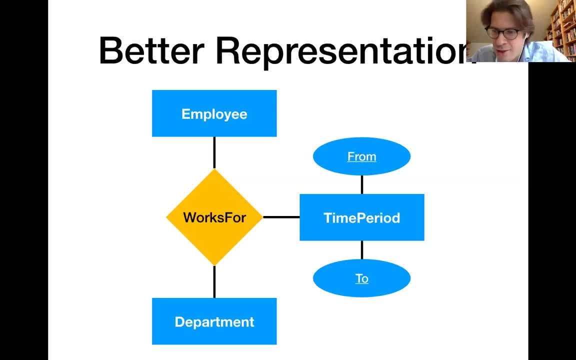 um with the time period. I assume that's the proposition here. So a priori, in this context you could also use aggregation. I imagine that you, via aggregation, that it works for relationship, has a time period, So in this scenario you could also model it. 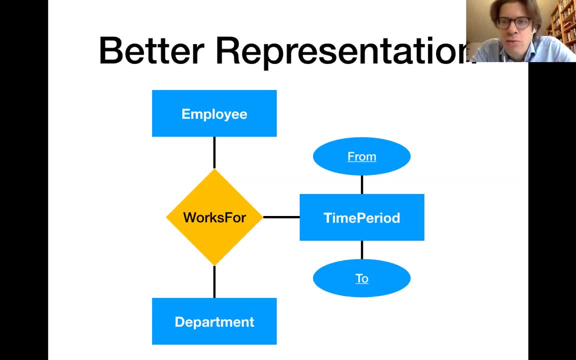 via aggregation. I assume that you would connect the works for relationship to a time period entity again perhaps, which would also be a possible. I'm not sure whether it gives you additional things that you can express in that way, that you cannot express in this way. So, with the corresponding constraints, I think you would get. 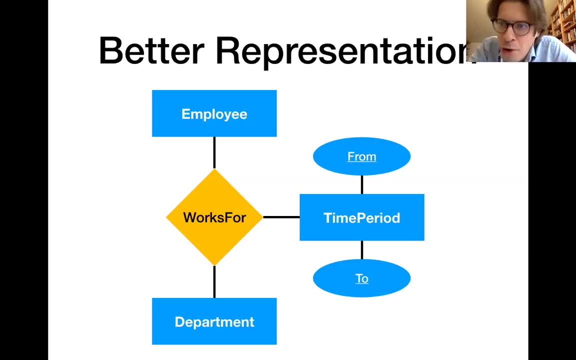 something which is close to what we are modeling here. So the answer is yes, you can use aggregation and the question is okay. so you want to make sure that the works for relationship has a time period. So in this representation that is actually ensured, because each of those works for 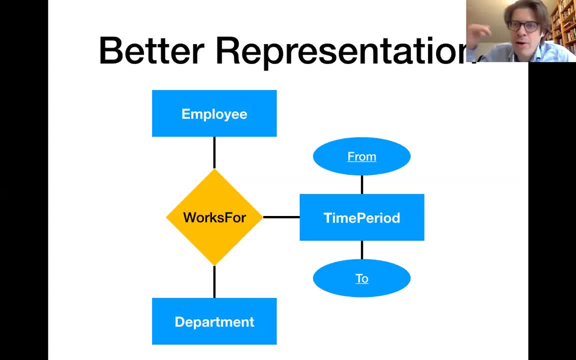 relationships must connect one employee, one department and one time period. So with this representation, you essentially ensure that we mark down the time period for the employment. All right, And then All right. and then there is another question: How can you make some of these relationships more explicit? 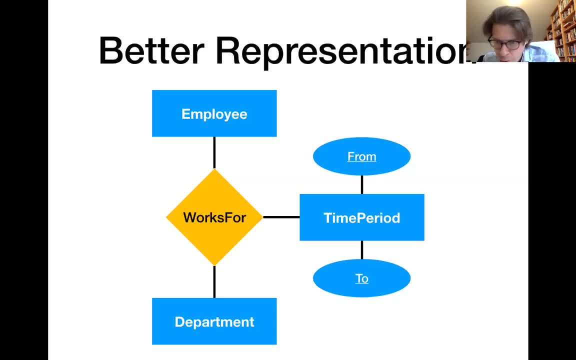 What about when things aren't as clear? Say, if an employee works for another employee in the department is a property of where they work. So this is a very good question. I think it's a very good question. I think it's a very good question. 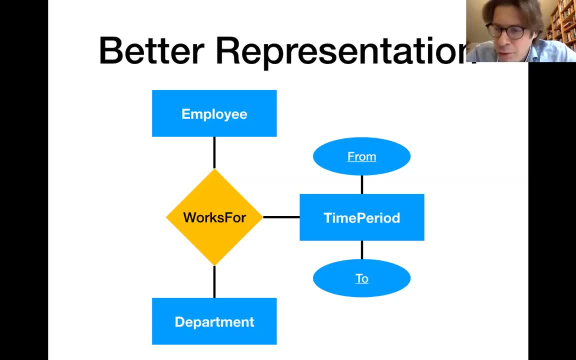 OK, So in general. so I mean, what we ultimately want to do with those entity relationship diagrams is that we essentially want to formulate those SQL, create commands for different tables in order to create a database schema into which you can insert your data. So it is true that it can sometimes 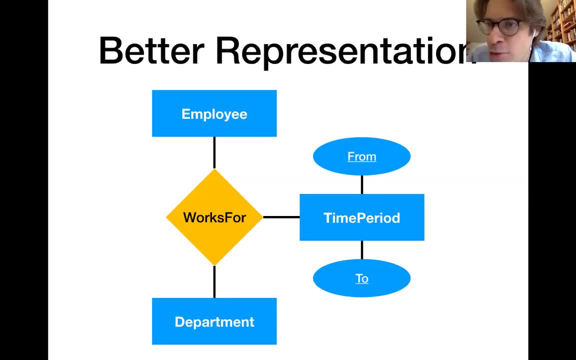 be challenging to consider all possible situations in advance. Often those database schemata, they need to evolve, They need to get changed over time in order to either extend them or in order to represent changes that a company is going through, for instance, which impact the data model that they want to use. 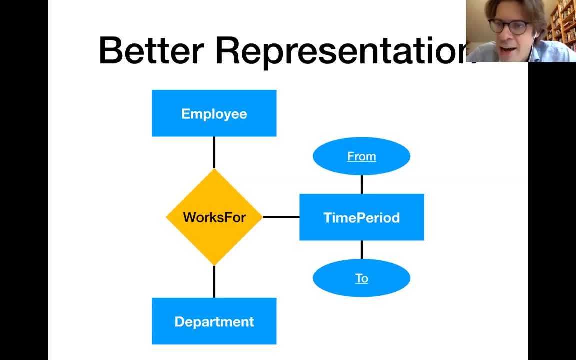 But I mean OK In principle. so basically I mean, if you want to work with a database, then you have to make a decision about which schema you want to use. You can, of course, adapt that decision over time. 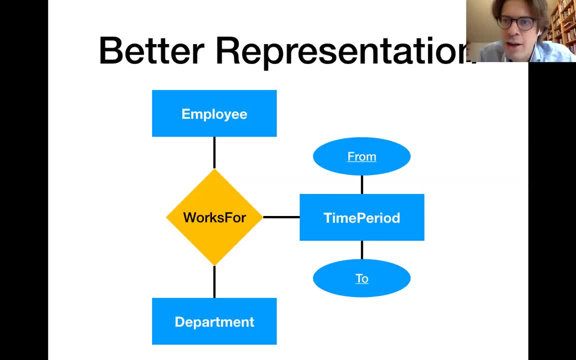 but you need to decide which tables to create. So entity relationship diagrams they help you to make that decision. But if your question refers to whether it can be difficult to integrate all possible situations in those entity relationship diagrams, I agree with you: That can be challenging. 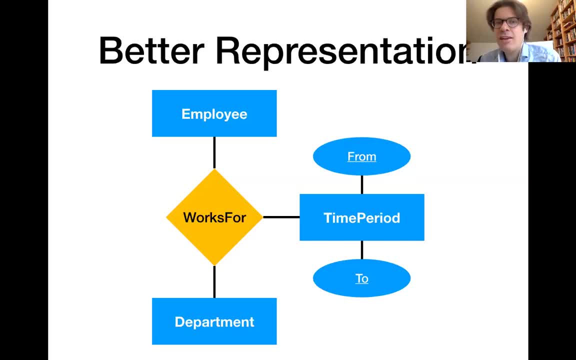 But for sure, if you want to work with a database, I mean you have to decide on the schema that you want to use in your database. So, even though it can be challenging, there is no alternative, basically, So OK. 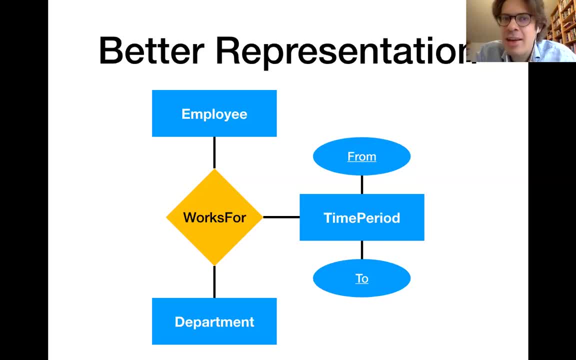 Yeah, But great question. So I mean, I think in many of those cases it is difficult to come up with a good entity relationship diagram. It's also an iterative process. You make a first graph, then you realize: oh there's. 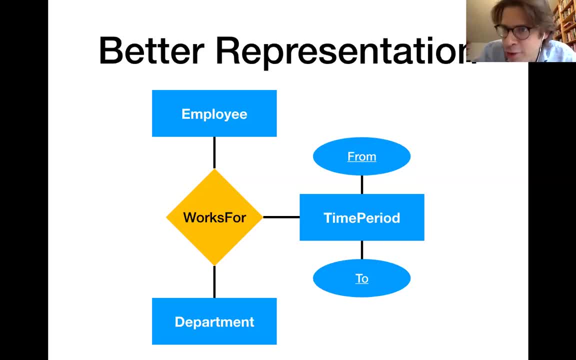 a situation that I didn't consider and which I cannot represent with this entity relationship diagram. Then you refine it and you do it a couple of times until you come to something that you like. So it is challenging, But I mean we have to decide on some structure for the database. 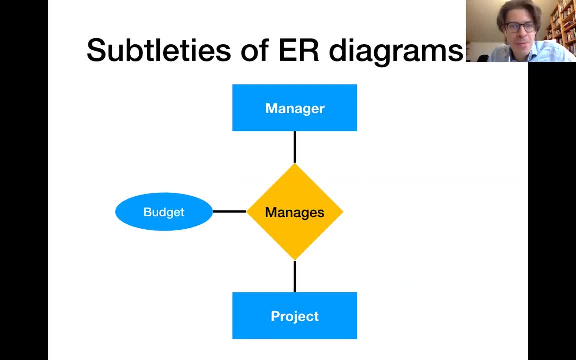 So it's not just because of the database, but because of the ecosystem, And that's just one example. We have to think about how we can make our database better, And there's a lot of things to think about. We have to think about how we can make the database better. 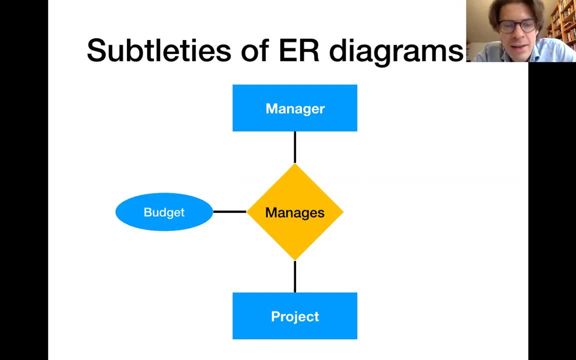 And then we have to think about how we can help the database to be more, much more efficient and more efficient, And that's really important. So that's the third one, the five questions. OK, Great, Great question. All right, Great questions. 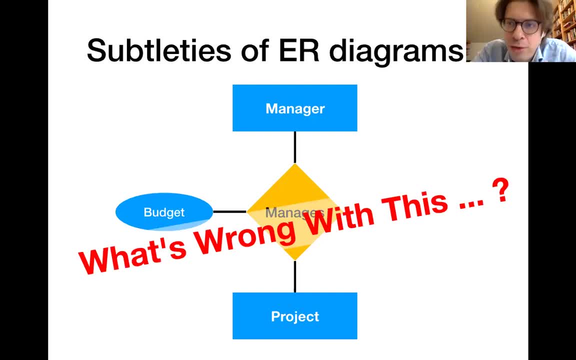 Now let's discuss a different scenario. Can anyone tell me what is wrong with this representation? OK, so there is some information that is not represented in this diagram. I mentioned that the VJ that is specific to one specific manager, but here it doesn't. 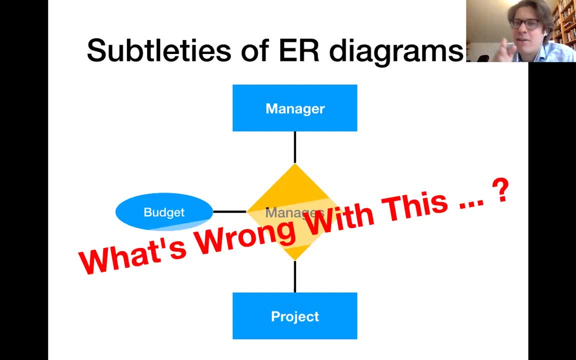 say how that VJ is partitioned across different projects. Yes, exactly, If one manager could manage multiple projects. yes, So I think, yes, So this is all aiming at the right thing. So the problem is this budget relationship And very correct here the point that one manager could. 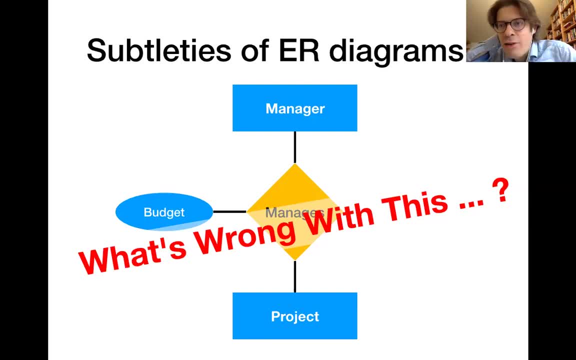 manage multiple projects And in that case, first of all, we are missing. We are missing information. so because we don't represent how the budget is partitioned across multiple projects And also we introduce some redundancy, Because I mean here we essentially 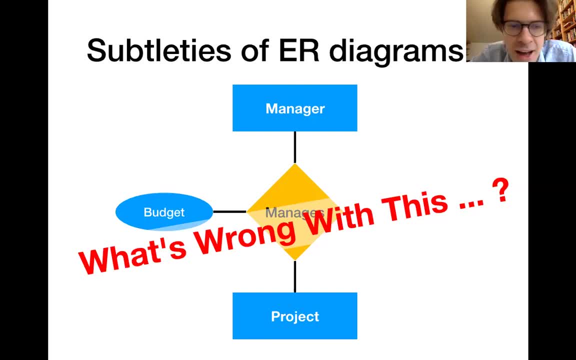 model, something that we would need to store this budget for each manager project combination, Those attributes of the relationships. they're essentially stored for each combination of the entities that are involved in the project. So it's an example of how these two parts of the relationship 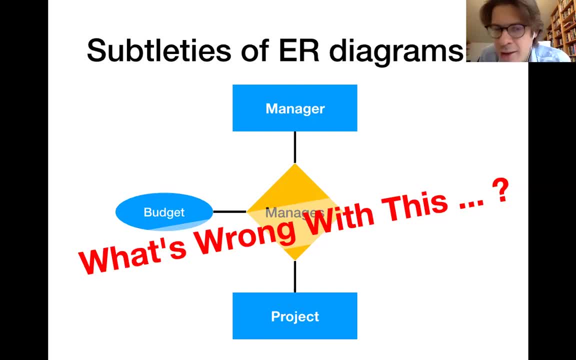 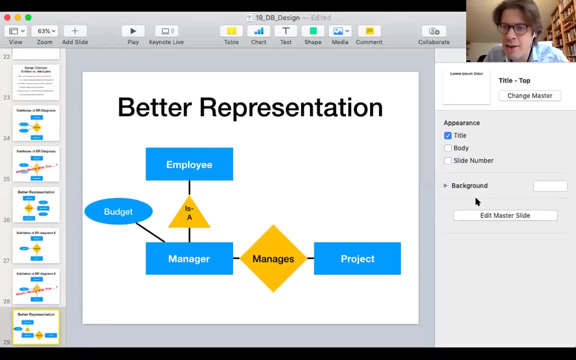 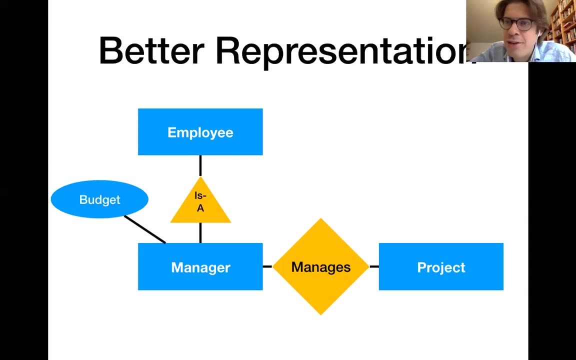 are working. So one manager has some sort of a management relationship, And if the VJ only depends on the manager but not on the project, then this representation is redundant. So a better way to store that would be, for instance, this one over here: 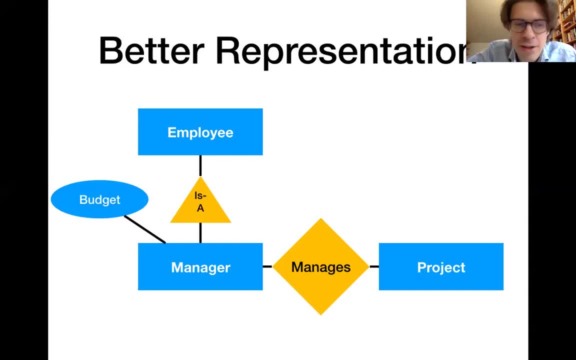 So here we represent managers as a specific type of employees that are associated with VJ. attribute is associated with the entity, not with the managers. relationship in that is more intuitive and avoids redundancies here. Still there would be. probably it would be. 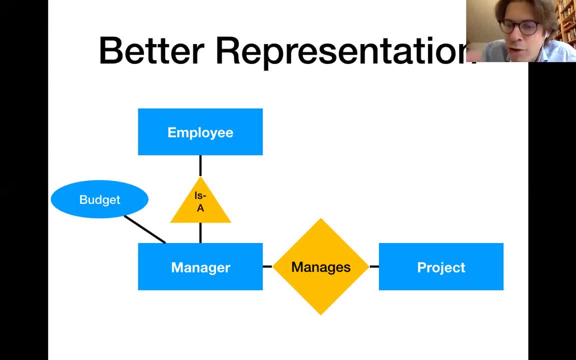 good to introduce the specific budget for each project and make this an attribute of the managers, a relationship. So that was a great point here. So here we have only taken care of the redundancy. So those are subtleties, But nevertheless, in practice it would be very important to make sure that you. 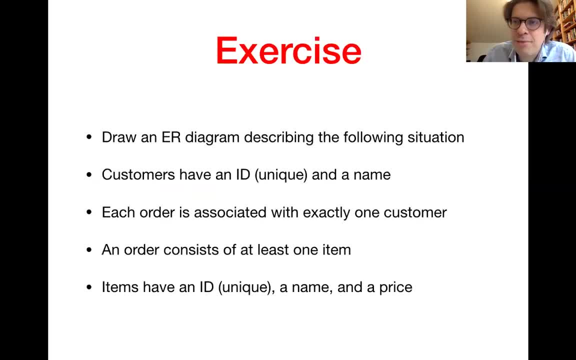 choose the right representation. All right Now, in order to get the hang of it a little bit, I wanted to make a little exercise. it gives you a couple of minutes. I tried to draw an entity relationship diagram which describes the following. 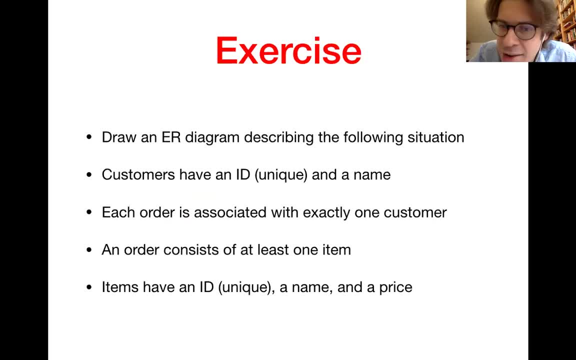 situation. So we are modeling customers that have a unique idea in the name. we have orders that are associated with customers And each order consists of at least one item. those items, they have also an ID which is unique: a name and a price. So 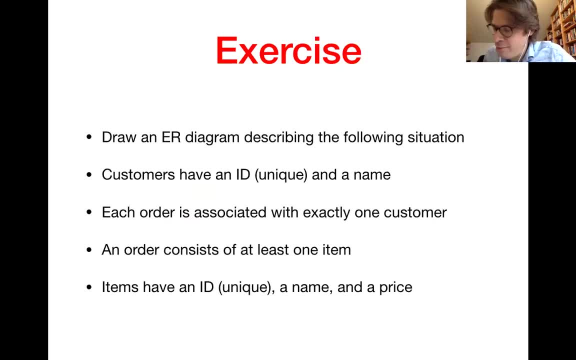 I give you a little bit of time to draw one of those entity relationship diagrams For this situation. So just take a sheet of paper, perhaps, and try to model that. If there's any more questions about entity relationship diagrams, I'm happy to answer them here. 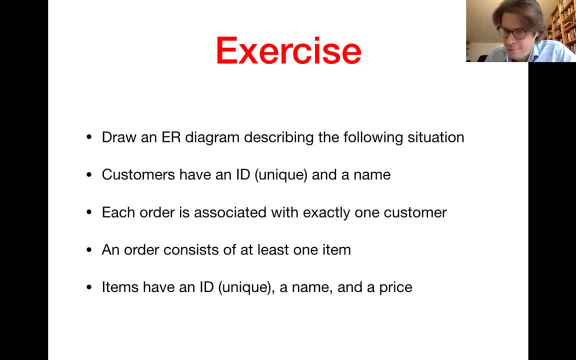 All right, All right, Thank you so much. Thank you so much for joining us today. We'll see you in the next session. Thank you so much for joining us and we'll see you in the next session. No questions on entity relationship diagrams. If you. 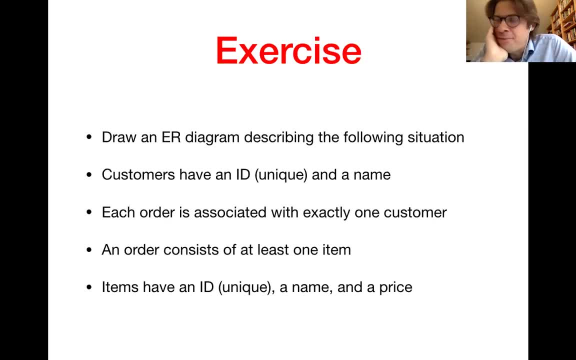 want one minute, then I'm going to show you the solution. All right, so let's take a look at that real quick. So here we introduce an entity type for the customer. We'll call it a label, And we'll talk about it a little bit later, But for now, 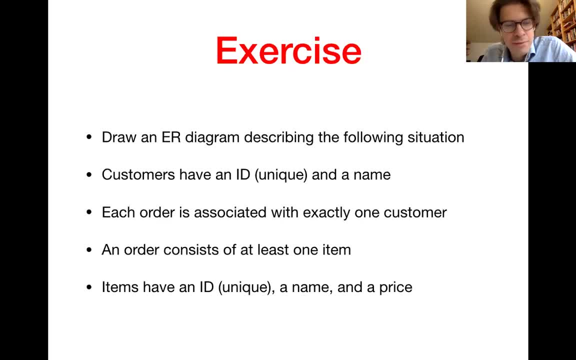 we're going to get started with the demo. So let's take a look at the demo And let's see if we can get started with the demo here. So we're going to show you the demo. So this is the demo we have created. So here we have our demo, So we can see what's. 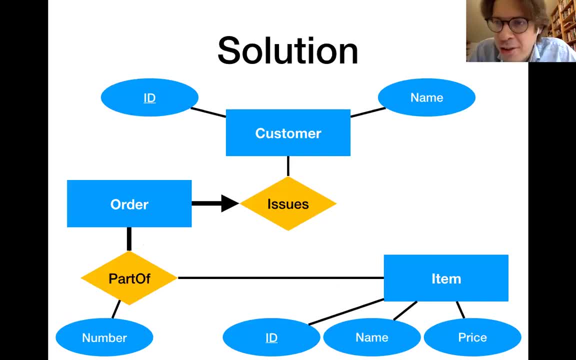 happening And let's quickly have a look. So here we introduce an entity type for the customer, So we have the demo here. So we customers with the associated attributes, which is ID and name- ID is marked as a key by underlining it, then we have a connection between customers and orders. 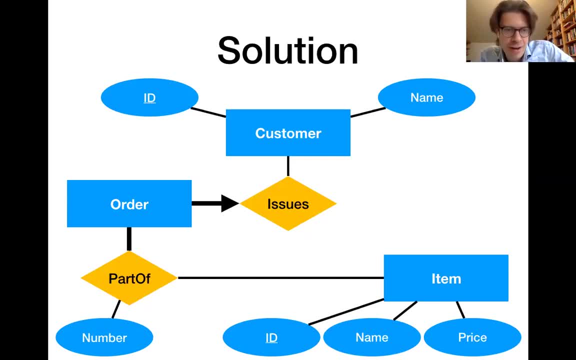 and we also have an association between orders and the items. items have the attributes that are mentioned in the description, and here the orders are connected to the items via a participation constraint. you have the sick line over there, which means that each order must consist of at least one. 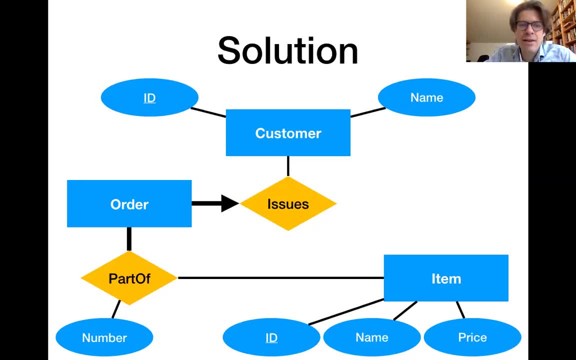 item. otherwise it is not a proper order. and since the part of a relationship connects us- specific orders and items- we might also have multiple items of the same type and in order to model that situation, we introduced the number attributes also between order and customer. logically, an order needs to belong to. 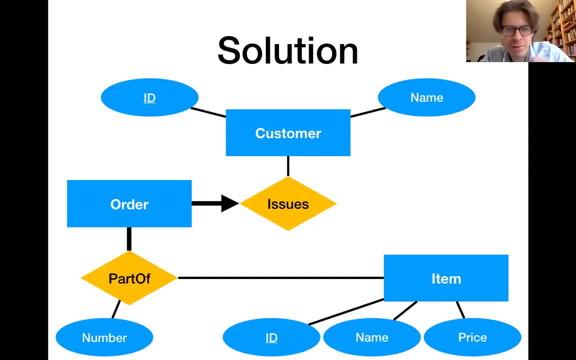 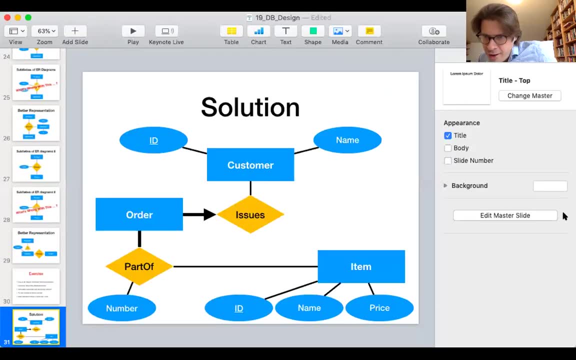 one customer, exactly one customer, and this is what the constraint here with the sick line and the error is expressing. and here is a question: is there a way to do this with order being a relationship instead of an entity? why not? so maybe one high level, a remark? so, in general, 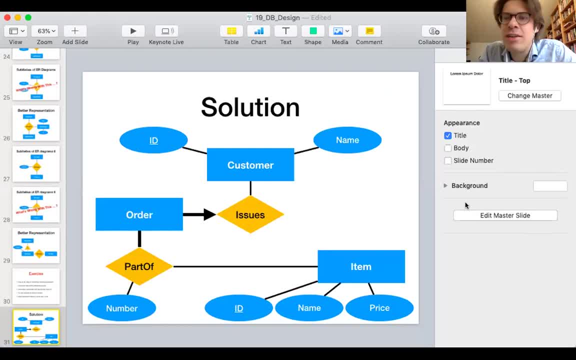 there's order, then there is no order given. the third sentence is just a always many possibilities to describe the same situation with entity relationship diagrams. So if there is a different solution from this one, it does not at all mean that that solution cannot be correct. 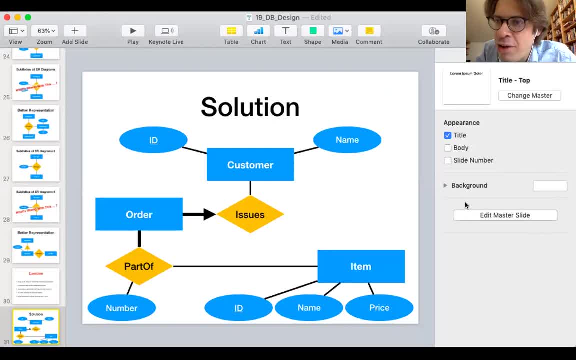 So, like when writing SQL queries, there's always many different ways to express the same query or express the same situation, And all of them can be correct. So modeling order as a relationship, So I assume that would be a relationship connecting the customer with items. 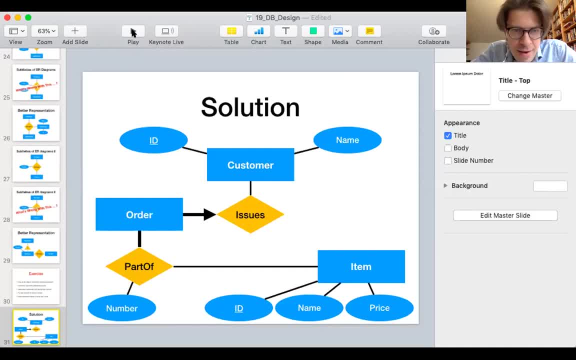 OK, And then, yeah, I think you can also make that work. So you would have to express that each item needs to be associated with an order. yeah, So, OK, I can see that It depends on the specifics, But I believe that there's also ways. 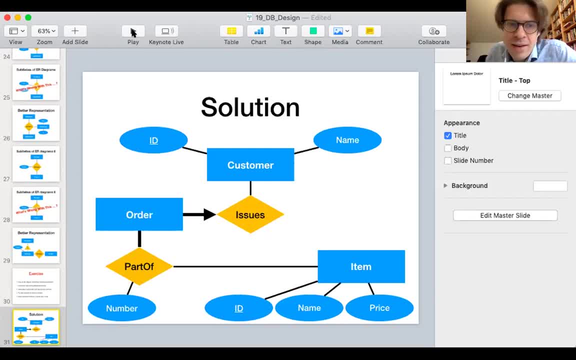 to model this when connecting customers and items with an order, relationship And number. that is an attribute of the part of, say, a relationship. So here those relationships essentially can contain information about each order and item combination at most once. So if you want to model the case that we 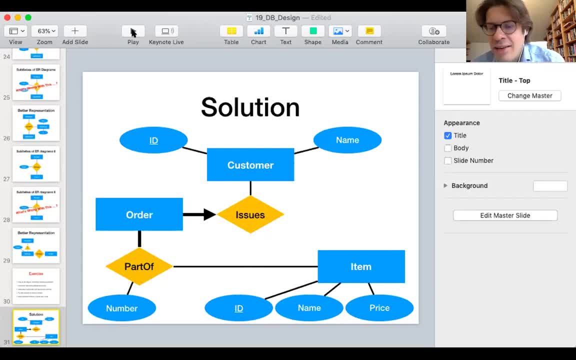 have multiple instances of an item in the same order, then the way to model that is to introduce an attribute which captures the number of items for each order: item combination, And so this is what we're going to do. OK, OK, OK. 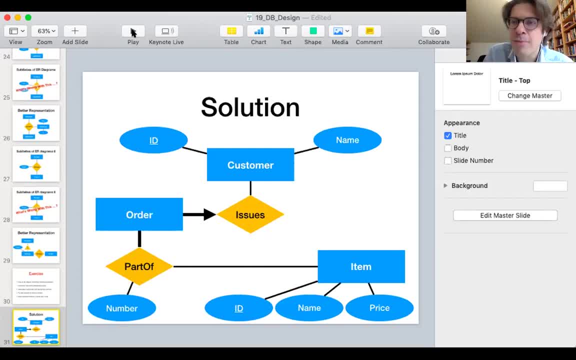 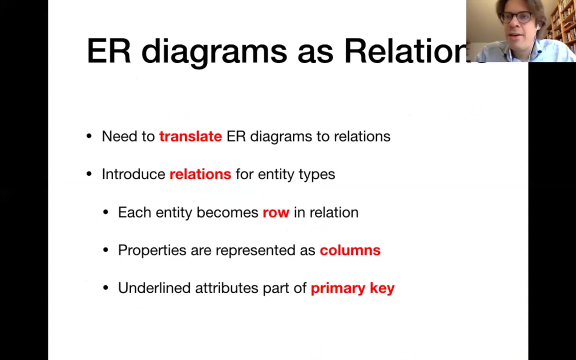 OK, OK. So essentially this is kind of what the diagram is essentially doing. So that is essentially the number of times that each item appears in an order. All right, So now we have learned formalism to represent a data, the database: 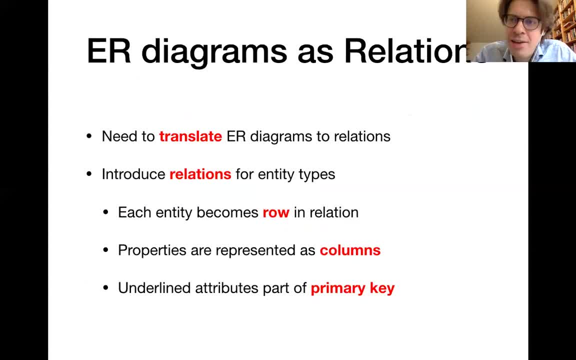 of abstraction, those entity relationship diagrams. Ultimately our goal is to translate them into SQL commands for creating the associated tables. So in the following we're going to see how we can translate those entity relationship diagrams into actual relations And then for those relations it is relatively natural. 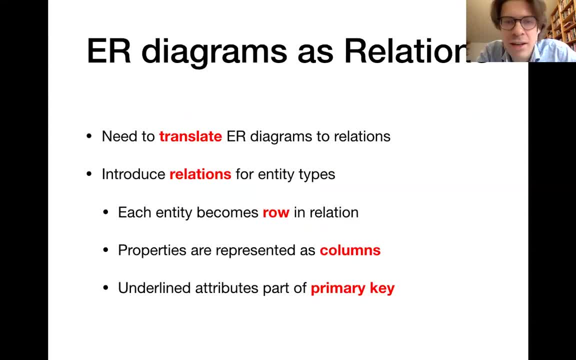 to formulate corresponding SQL commands for creating those relations. So in order to represent those entity types which appear as rectangles in the diagrams, we introduce a relation such that one entity corresponds to one row in that relation And different properties of an entity are represented as columns of that relation. 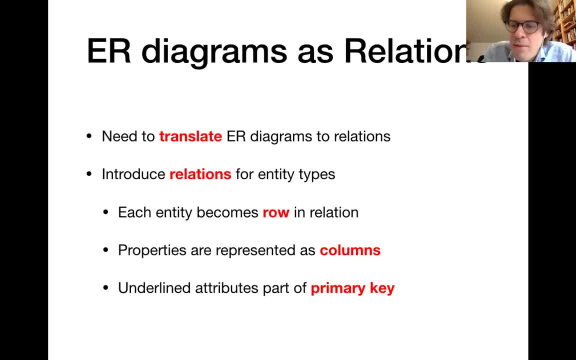 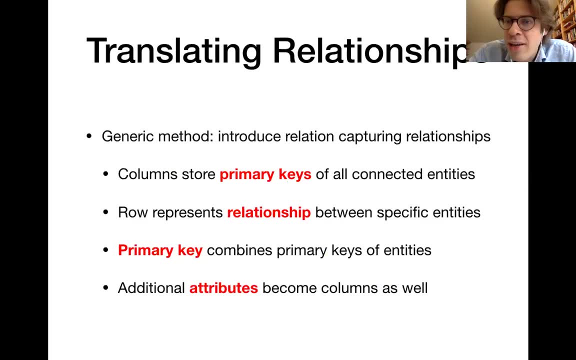 The underlined attributes, they become the primary key For relationships. we can also introduce relations which essentially contain one row for each combination of connected entities. So the columns of that relation representing the relationship, the diamond in the entity relationship diagram, would essentially contain the primary keys of all the entities. 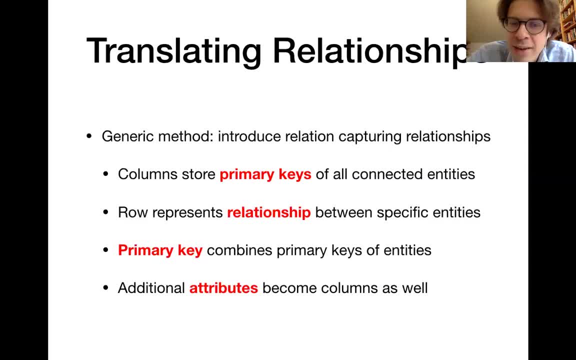 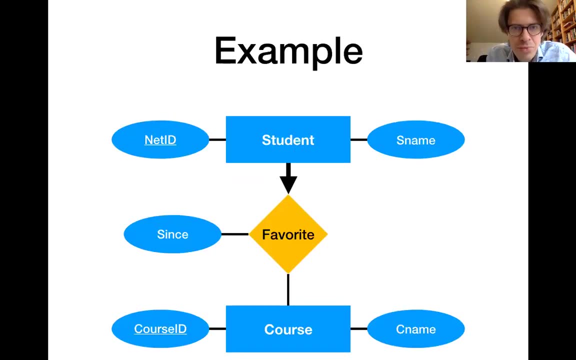 that the relationship connects, And then one row would represent the relationship between, for example, the student and the student. If the relationship is associated with additional attributes, then those attributes become additional columns in that relation. Let's make things a little bit more concrete by an example. 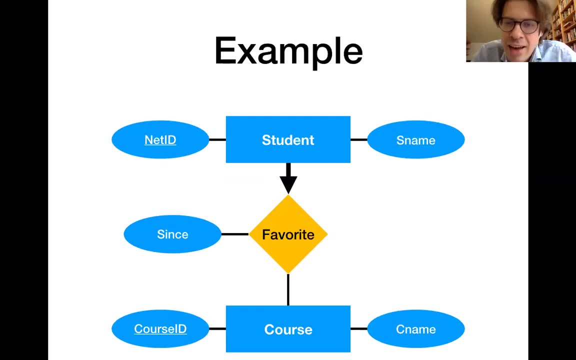 So here we have a relationship between the students and the courses. We are expressing that each student has exactly one favorite course. We have the net ID and the student name as attributes of the student And we have the course ID and the course name as attributes of the course. 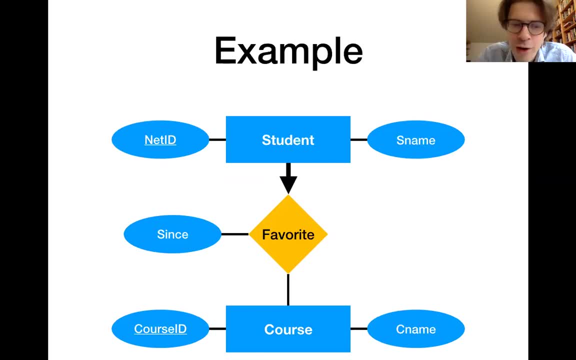 And also this favorite relationship is associated with one attribute, since, So for a specific combination of a student and a course, this attribute gives us the time starting from which the course became the favorite of the student, And now we can chat, And now we can expand. 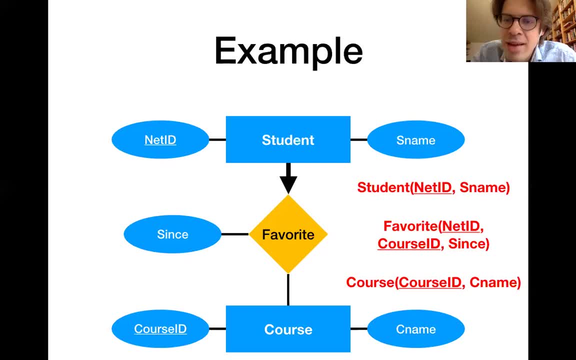 And we can translate this entity relationship diagram into relations, as you see here in red. So the student entities they get translated into a relation: a student which has columns for the net ID and the student name And the net ID is the key column which. 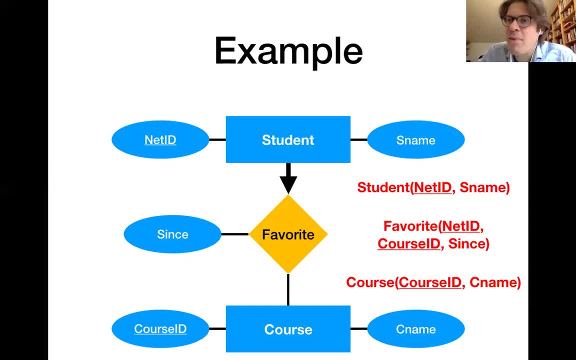 when representing relations, we always represent that as well by underlining The corresponding column. On the other side we have a relation, a course which stores the courses And again has course ID as a key column, And then the relationship between the students. 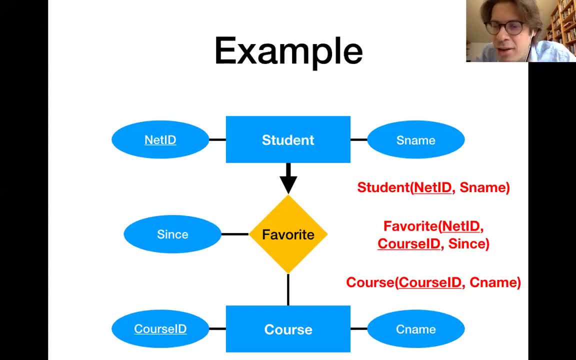 and the courses is expressed by this favorite relation which has the net ID and the course ID as the primary key columns. So here this is essentially the combination of the primary keys of all involved entities And also it has this additional column in order. 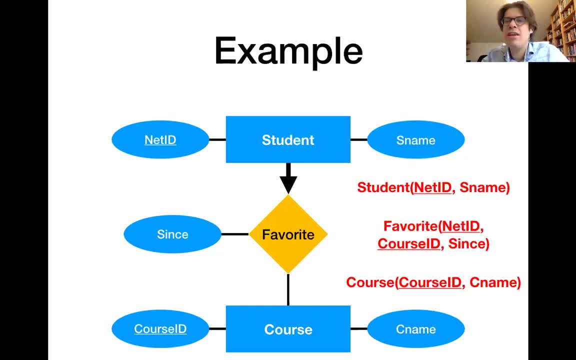 to store the since attribute. So here that is one generic way in which we can model relationships, how we can translate them into actual relations. Here we can just add one corresponding relation And the primary key columns of that relation, just collect the primary key columns from all the involved entities. 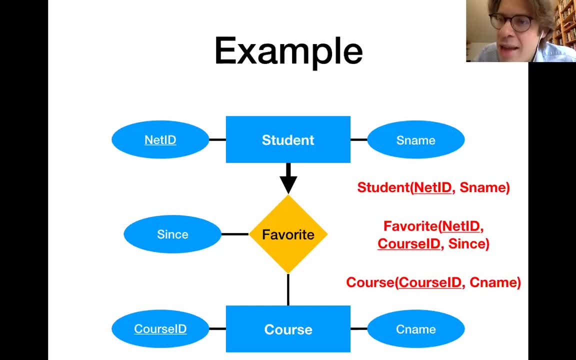 So we can store something about each possible combination of students and courses here, And then, after I have those relations, it is relatively natural to formulate corresponding, create table statements in SQL in order to actually get the database that this diagram is describing. Now I can do better than that, depending 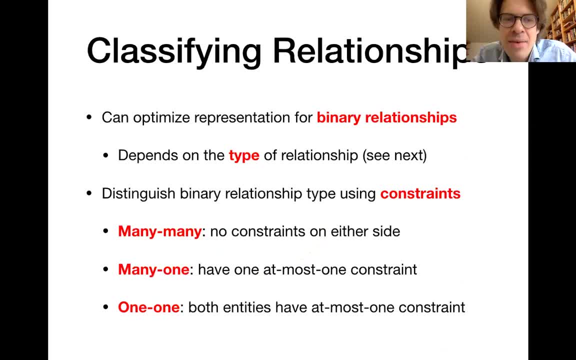 on the type of the relationship. I mean specifically for binary relationship. we have a couple of different types. We distinguish the type of relationship based on the constraints that I have and say that I can either have a binary relationship of type many, many, which essentially connects an arbitrary type. 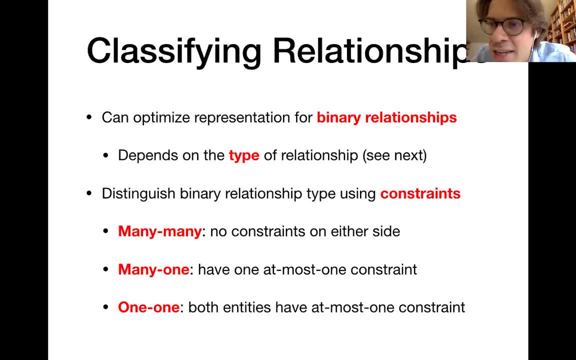 an arbitrary number of entities to an arbitrary number of entities on the other side. I can have a many to one relationship, which means that entities on one side can only appear once in this relationship, And I can have a one to one relationship, which means that entities on both sides of the relationship 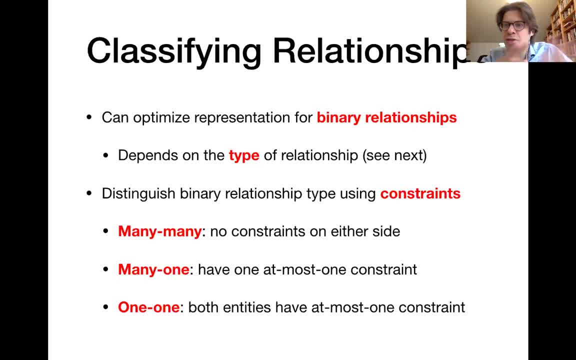 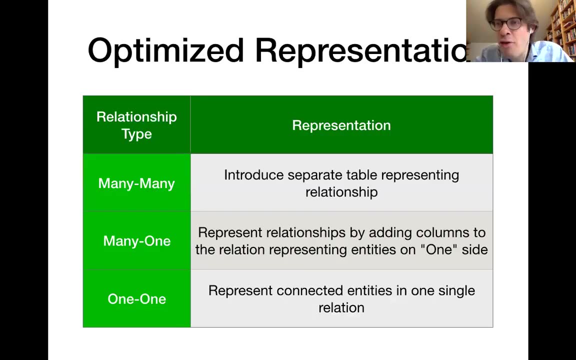 can only appear once within it. So I mean all of those different relationship types. they use at most one constraint that we have seen before, which is represented as an arrow in the entity relationship diagram, And this is a quick overview of how I can model relationships of different types. 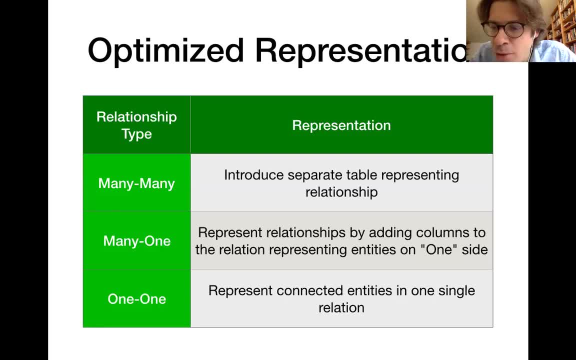 The many to many relationship is the most generic type of relationship because it doesn't impose any constraints on how often entities can be in that relationship. So here, the only way to represent that is the generic way where we introduce one new relation in order to represent that relationship. 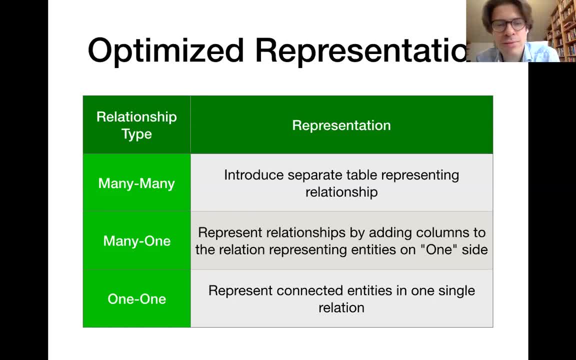 And that is the way which we have already seen before For the many to one relationship. we can essentially avoid introducing a new, separate relation in order to model the relationship. Instead, we can merge the relationship and represent it as additional columns so that we have a one-on-one relationship of the relation. 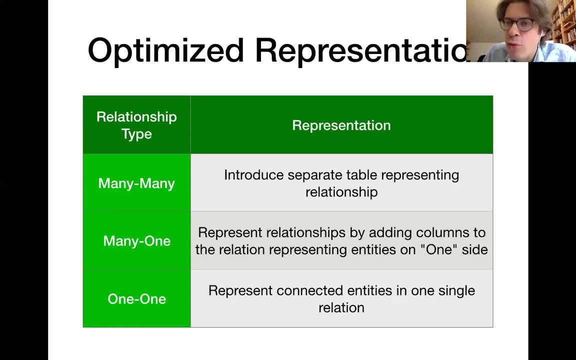 representing entities on the one side. If I have a one-on-one relationship, then I can even simplify things further and represent both entities involved in the relationship, together with the relationship itself, in one single relation, in one single table. Now that is a little bit abstract, so let's make it more concrete. 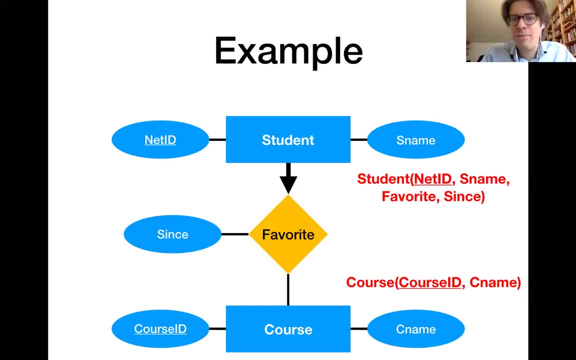 By an example here. So here we have the same example as before, And now in this case we have the constraint that a student can only have one specific course as a favorite. So here what we can do, is that so here? 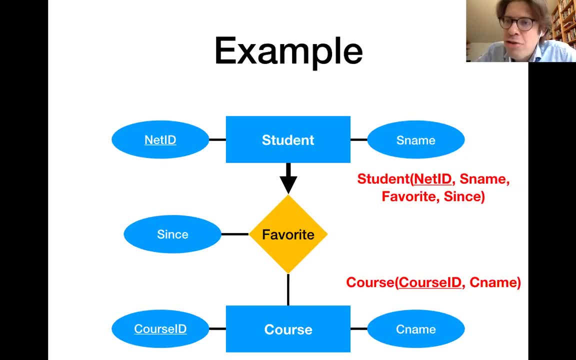 what we can do is that we introduce a new column in the student relation which points at the favorite course. So we have here again the net ID column, the student name column, But now we have essentially merged columns that we have put into a separate relation before. 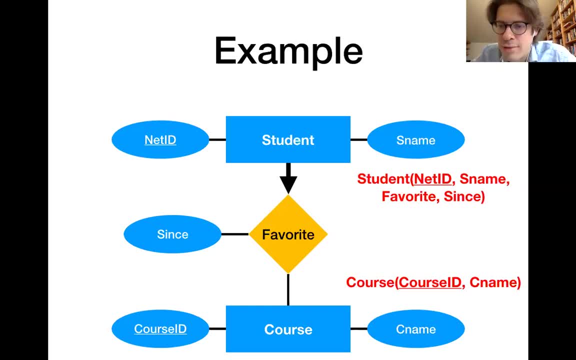 Now we have merged them into the student relation. So here we have the favorite, which is essentially pointing to the course ID of the favorite course, And then we also have the synth column, which represents the point in time at which the course became the favorite. 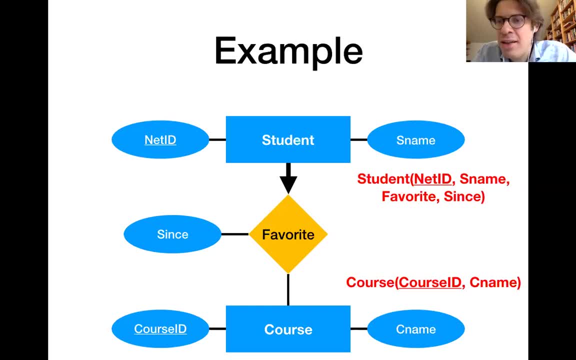 And we can only do that because we know that for each student they can be at most- or in this case, exactly- one favorite course. Because of that, we know that we can just put all of that information into the same row which describes the corresponding student. 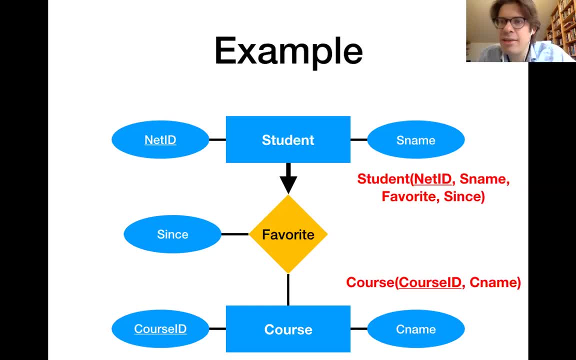 If a student could have multiple favorite courses, then the system would not work. In that case, I would need to introduce a new, separate relation in order to represent this relationship, And here we have another example. So here we have the connection between lecturers and courses.